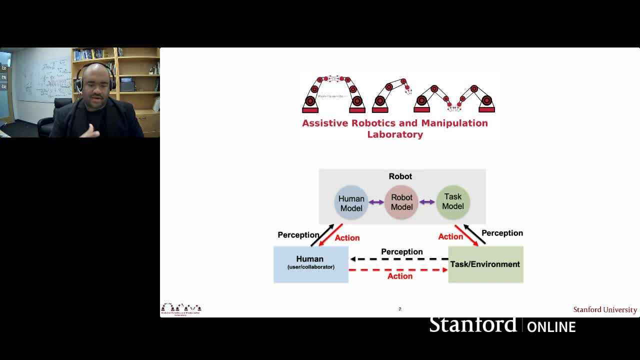 after robotic autonomy. So if you think about robotic autonomy, that's the ability for a robot to be in an environment to understand itself and its task and be able to complete that effectively. But what comes next is thinking about how that robot is going to be able to. 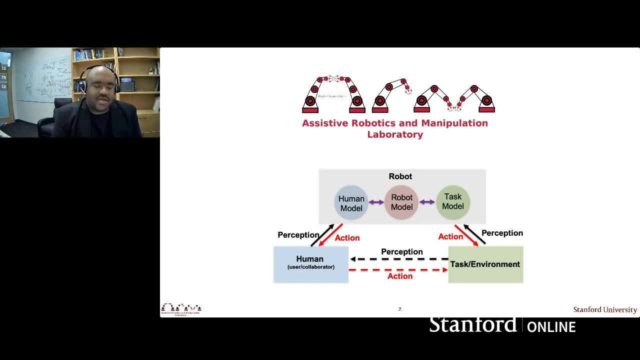 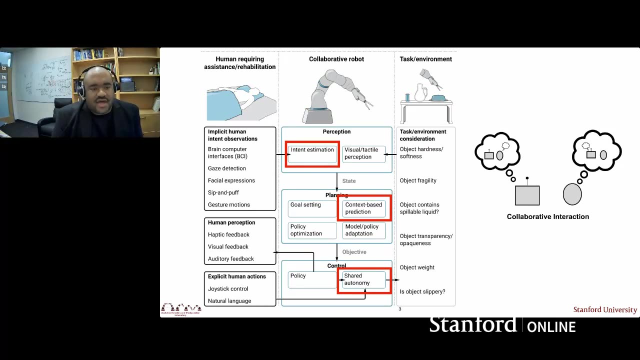 understand itself and its tasks and be able to complete that effectively. But what comes? thinking about how that robot might need to team with humans or other robots, And to do that effectively requires modeling those human teammates. I have this figure here, shown on the left, that 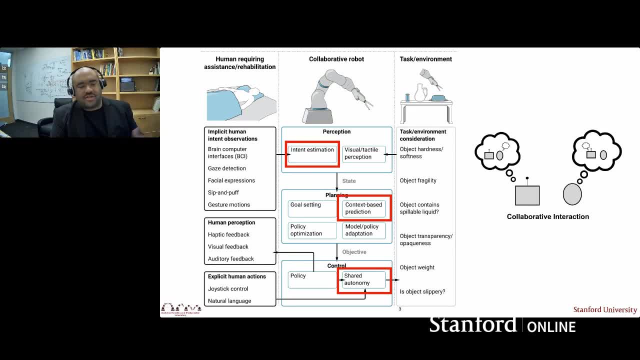 outlines how collaborative robotics fits into this larger conversation of robotic autonomy. So, when you think about the principles of robotic autonomy, a robot needs to be able to do three things. It needs to be able to see, think and act. Formally, that's perception. 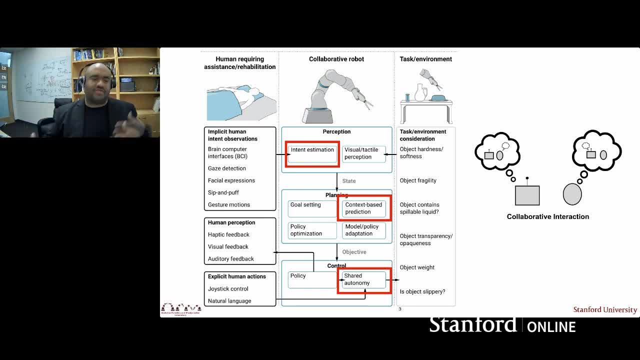 How do you observe the world? through a camera, through the sense of touch or other mechanisms, other sensors, And reduce this down to a state, which is a collection of variables that change And, based on observing their change, you can say something about how the world is evolving? 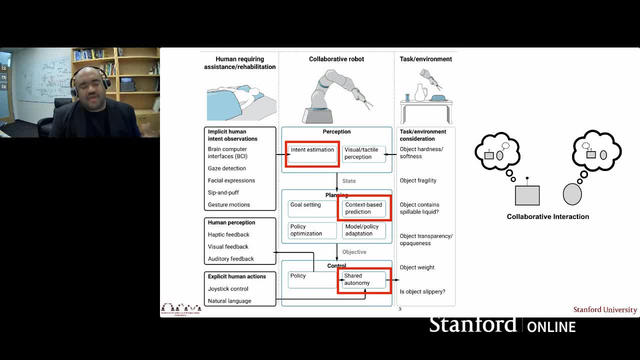 And then, given what you observed in your environment, how do you plan on what you want to do next in order to achieve some objective? And then, how do you control, How do you actuate yourself, How do you move, How do you provide some input? that 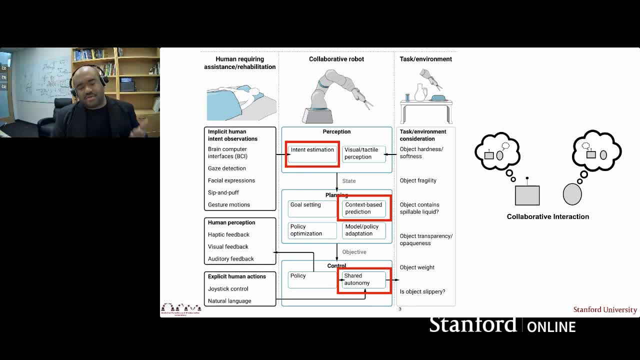 changes the state of the world. So that's the see, think, act, perception, planning and control In the larger context of how robots might be teammates. some of the perception may include observing humans in your environment. So how do you estimate their intent? 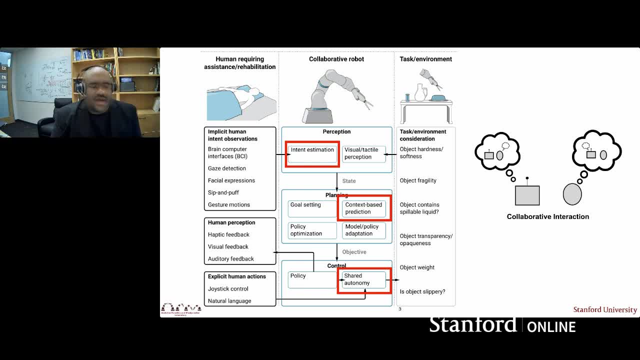 So something that's very popular nowadays are language models, And that's a very adequate way to obtain intent from those around you. So perhaps I can speak to my robot and say: hey, can you pick up this cup of water on the table? 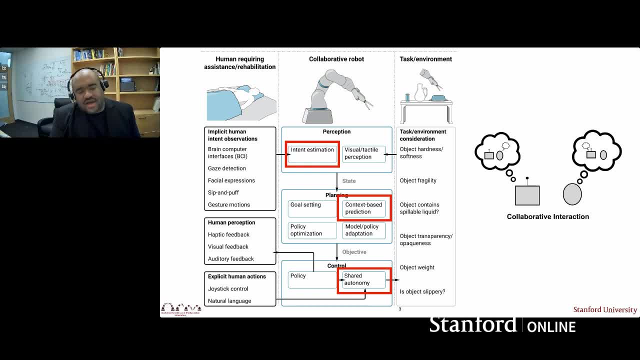 And maybe that is a valid form of input. But in my lab and I think another interesting question is, when things have to move very quickly, it's sometimes not always efficient to have to use sentences to describe what you intend, And I would postulate to you that when 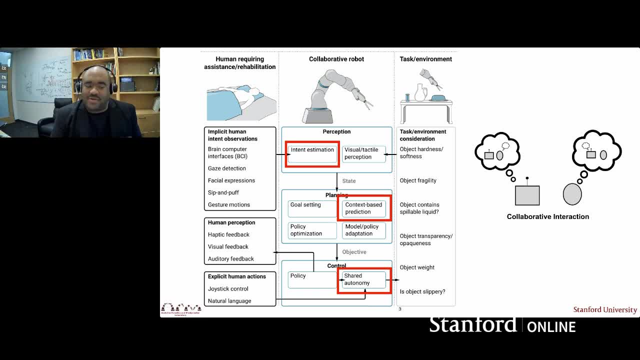 humans work together. we also don't always use language. Maybe we use it a lot, But we don't always use language to convey our intent, And one of my favorite examples is particularly in sports. So if you have people working together in sports, 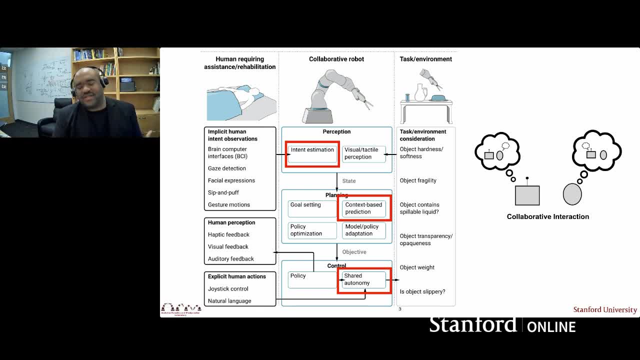 take soccer or basketball. they spend a lot of time working together, practicing, So they understand again how they want to achieve their objective, like scoring a point, But they're very familiar with the abilities and the signals that each other are able to convey. 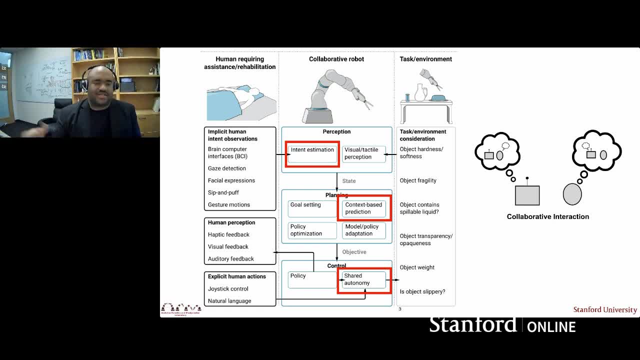 And so, given the abilities of your teammate, you can exploit that to actually, for instance, score a goal. And so the ability to understand your teammate, to be able to predict them, to be able to read them, is crucial as a tactical advantage in sports. 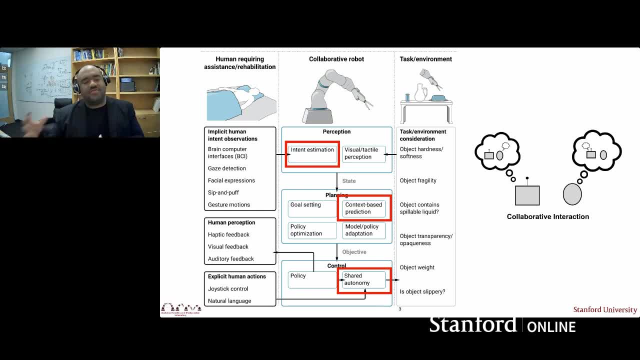 And this notion of how do you estimate what your human teammate would need if you're a robot is what we're trying to capture And we need to express that mathematically And that's what we're going to get in today. How do we express that mathematically? 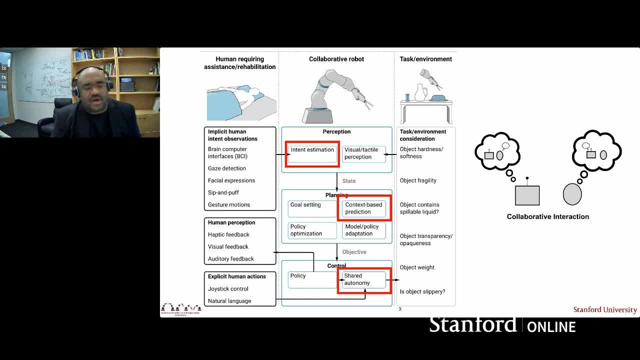 So I've highlighted here on the left-hand side three of these main points in red which we'll touch on in more detail. The intent estimation: how do I observe a human and pull out a state that allows me to estimate the variables that are changing? 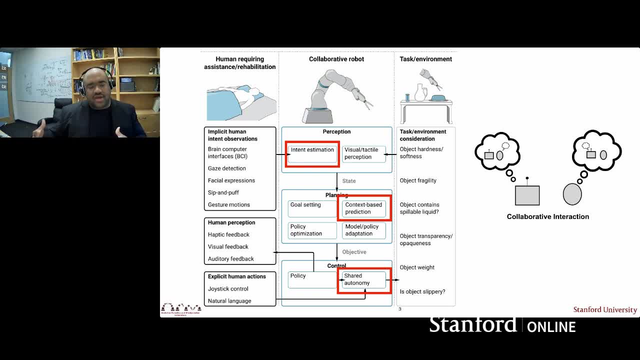 How do I use that state and knowledge of the tasks that we're trying to do together to predict how my actions may influence the human and how their actions may influence me? And then, with that prediction, how do I choose what actions I should take? 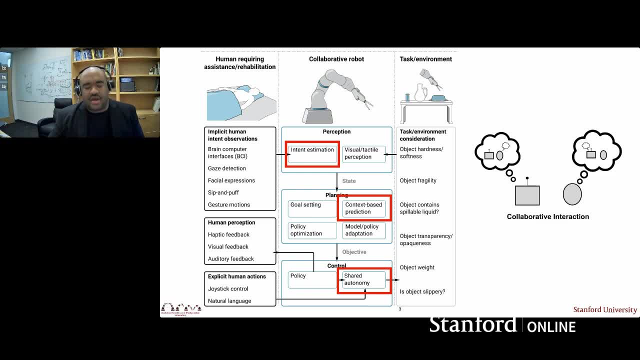 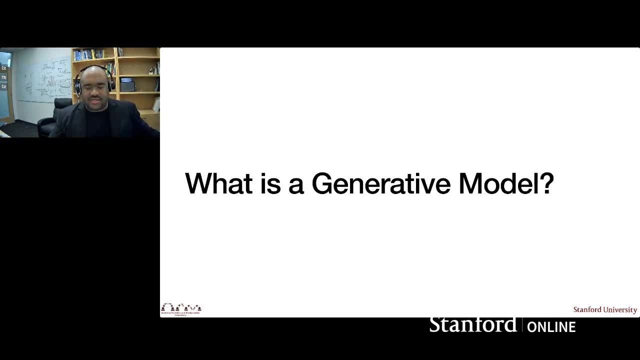 That will lead to a better outcome for the overall team. So, to start this conversation off, we're going to build some tools. first, We mentioned how do we need to mathematically model the ability to estimate intent. There are a few ways to think about this. 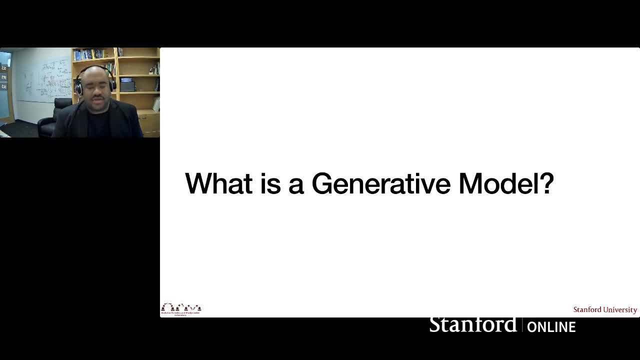 but the most popular way right now is through something called a generative model. This is not necessarily a new concept. However, some of the tools that are used to calculate it nowadays are very hot and very capable. And to start off here, I want to begin the conversation. 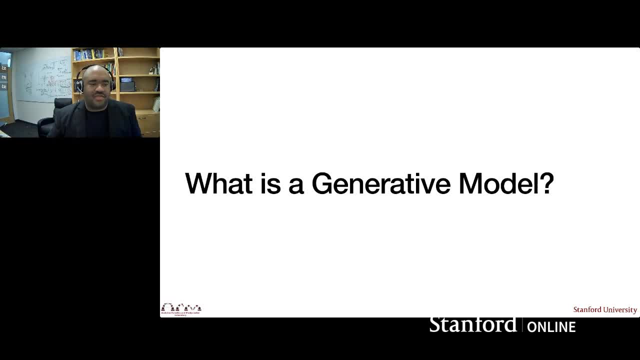 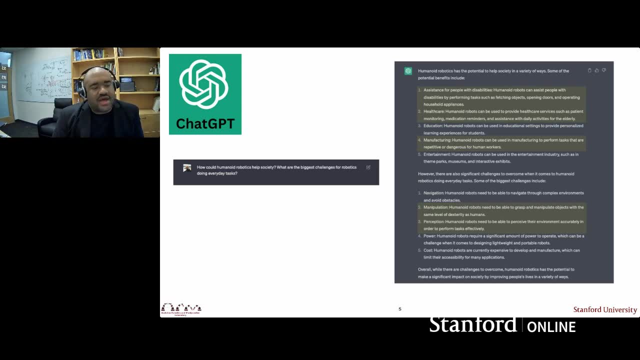 with a tool that most of you are probably very familiar with- ChatGPT- So I'm sure we've all had a chance to try this out. You can go to ChatGPT OpenAI, you can put in a prompt and you can get a very good personalized response. 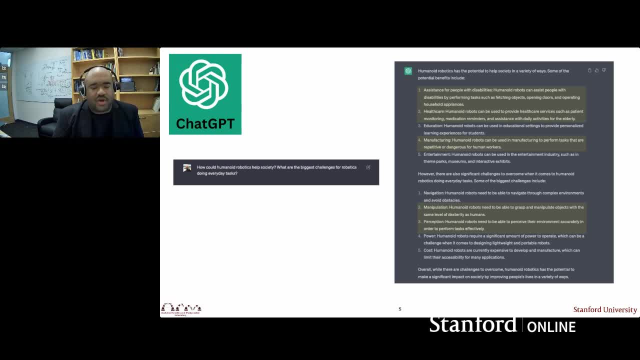 that most of the time is pretty much on point with what you might have inputted as a query. So here is an example I've put in here: How could humanoid robots help society? What are the biggest challenges for robots doing everyday tasks? 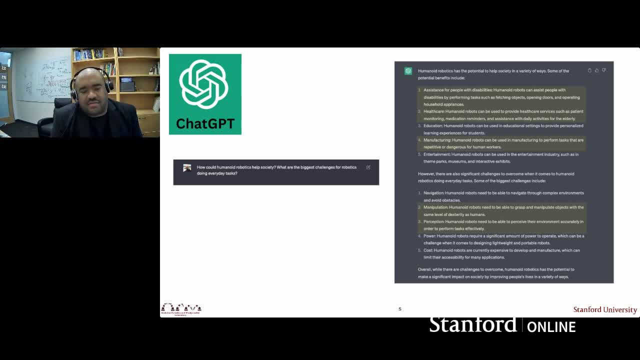 And some of these answers I completely agree with Highlighted here. on the right, you can provide assistance for those with disabilities, There's health care. manufacturing, manipulation and perception are the challenges. Did a very good job of pulling That answer, very realistic on point. 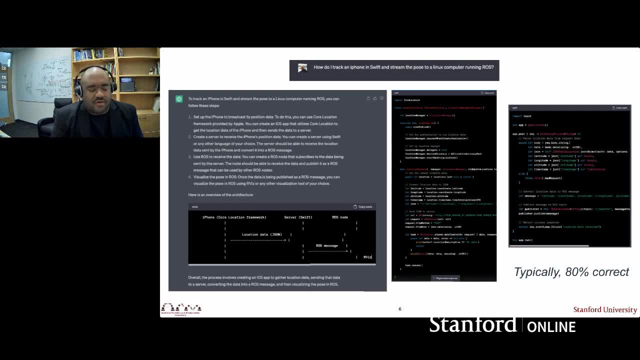 Beyond that you might see applications of for actual technical assistance. So let's say you have a wearable sensor where you want to use an iPhone to do some sort of pose tracking of a camera as you walk through a particular space. You can ask how you might use camera data from the Swift. 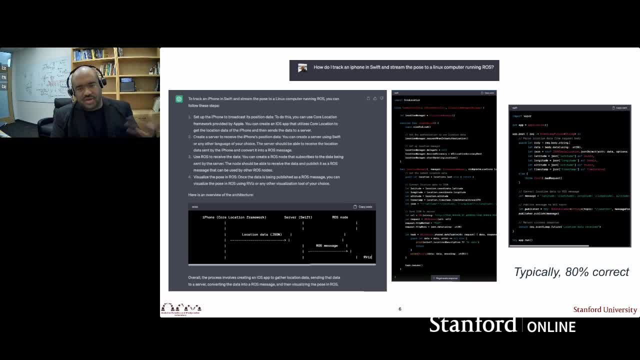 which is the coding platform for Apple, to stream that to a computer that you might connect with other robotic components through Linux and ROS, And then you can see that this can give a really good output. That again is typically about 80% correct. 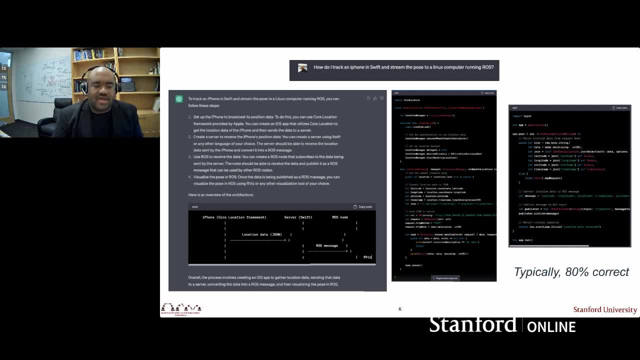 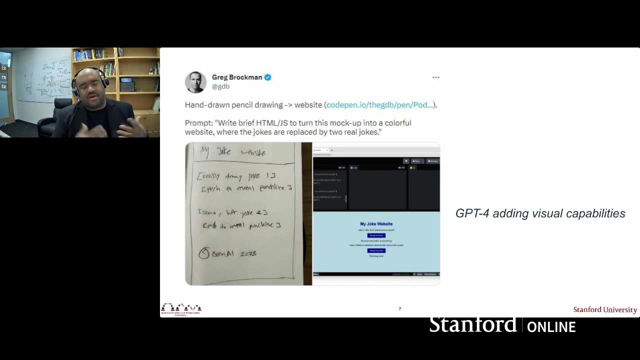 So if you kind of know this general coding structure, this can really get you moving in the right direction quickly in order to begin implementing these strategies. And, of course, with GPT-4, you have the ability to take a picture of some website. 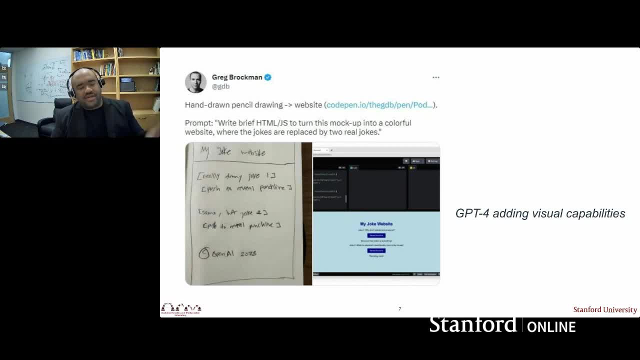 Or input, And then it can actually take a picture, a rough idea, and correlate this here to actual HTML code and other things like this. It can use images to also generate text. So what's going on under the hood here And what are some domains for this type? 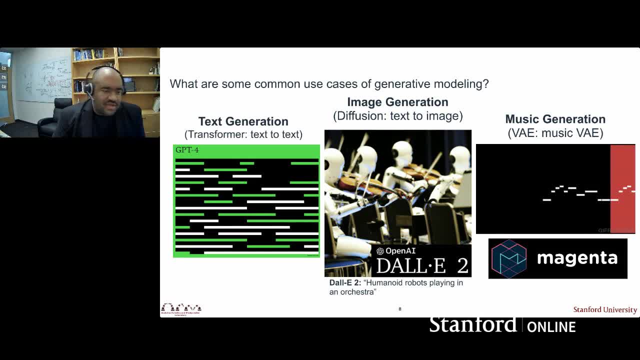 of generative modeling. So some of the examples I've given you just now include text generation: You put some text into this model and text comes out. Diffusion, image generation: you can put text in and an image may come out. 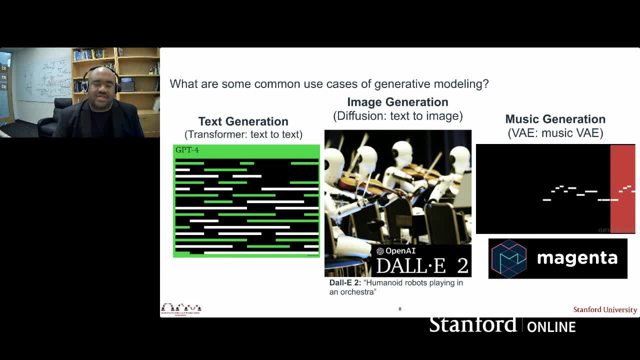 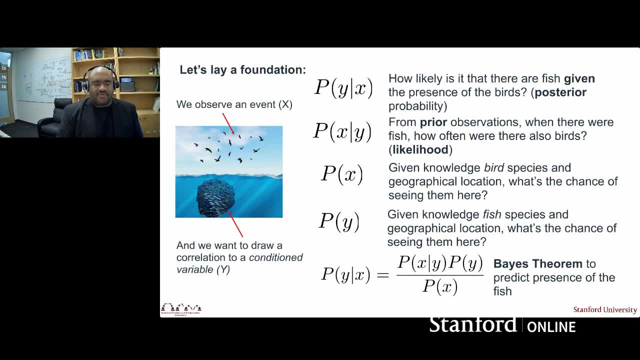 And even music. You can put in music signals and music will actually come out with these different tools. But before we get into them even more, I'd like to lay a very high-level, quick mathematical foundation, And I find that this example here is very digestible. 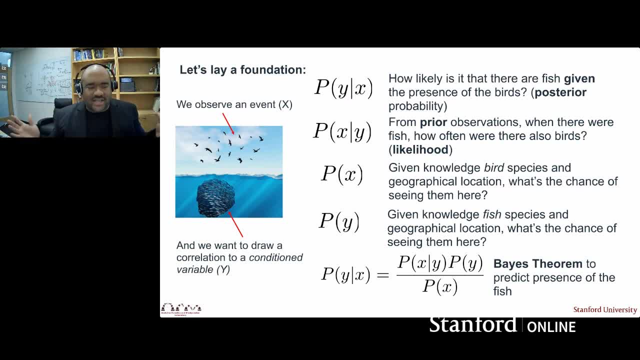 So I would like to invoke your imagination. Imagine you're a fisherman And you're trying to determine where you should sail your boat to find some fish, And you notice from past experience that it might be helpful to determine where the birds might be flying to actually drive. 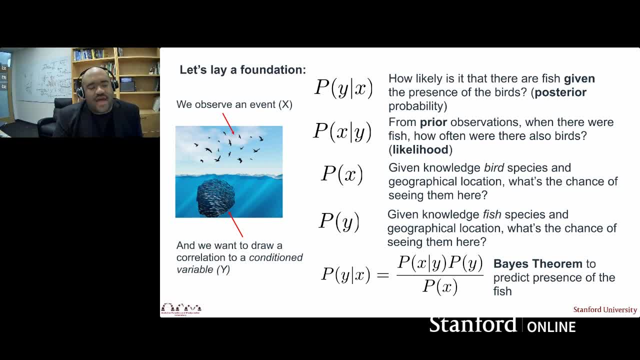 your ship to that relative location. So here on the left we see our birds. I'm going to call them an event x. the presence of the birds And the fish that are under the water will call this variable y And our goal. 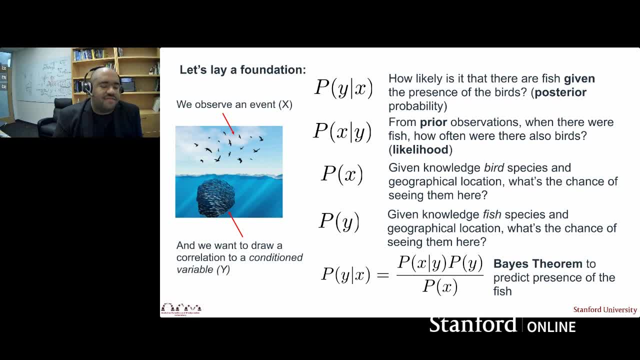 Is determine the relationship between the fish under the water and the birds that are in the air. So please excuse the fact that this is all on one slide, but if you go to the very top line here we have this p of y and this upward line and x, and this is telling us what is the probability. 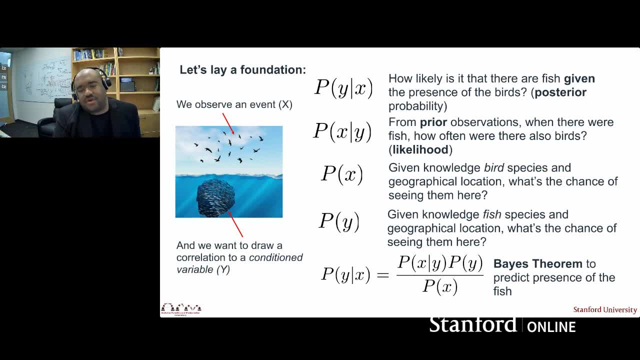 that we will see the fish, given the presence of the birds, and we'll call this a posterior probability. And we can find this if we know a few things, statistically, If we can say from prior observations: we've seen in past data, past experiences, that when there were fish, how often 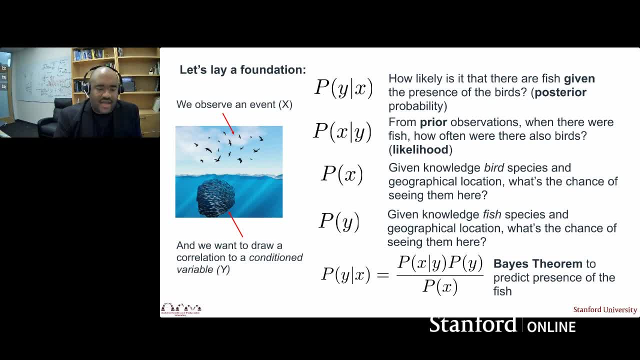 were there birds? that will give us p of x conditioned on y. What is the likelihood of birds, given there were fish? And then if we have some fundamental knowledge of the species? so what is the probability that the bird species is going to be in this geographical location? 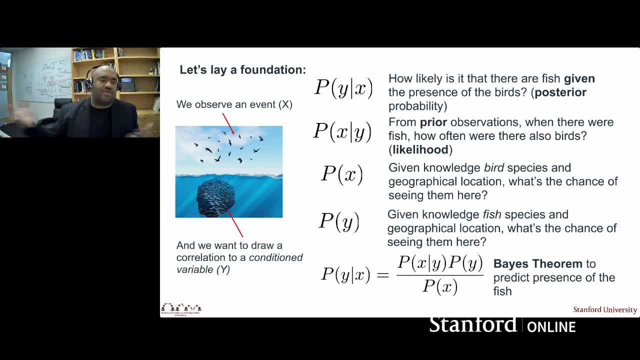 Given this time of year, have they migrated Or what's their likely presence of being there? Because there could be fish and no birds? simply because the birds have migrated. And likewise for the fish there could be birds. but if the fish migratory patterns are known, then we can use. 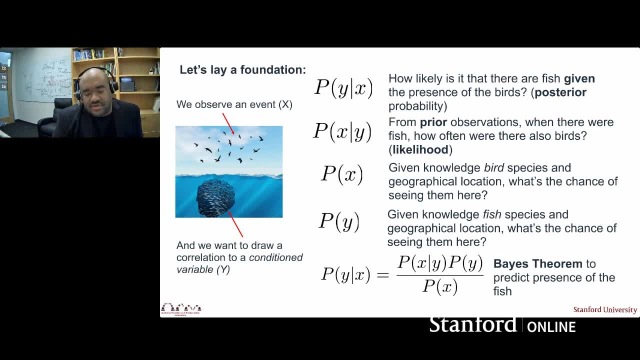 that knowledge as well. And this leads us to a very fundamental equation in machine learning, which is Bayes' theorem, where effectively we can use this prior information about how birds and fish relate and the fundamental knowledge of those species to then calculate. 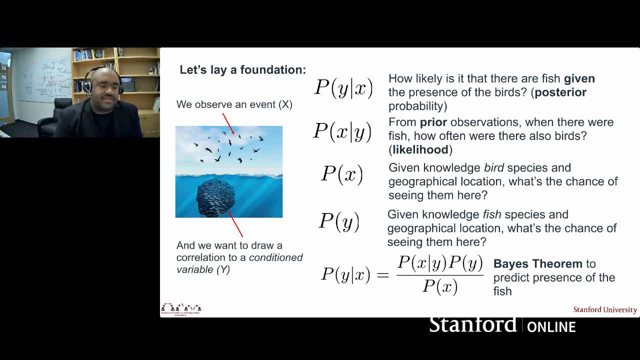 this posterior probability, What is the likelihood of seeing fish, given there were birds? Now I won't get too mathematical on you, but I wanted to give this foundation so that you kind of have a handle when we talk about these tools And Bayes' theorem is. 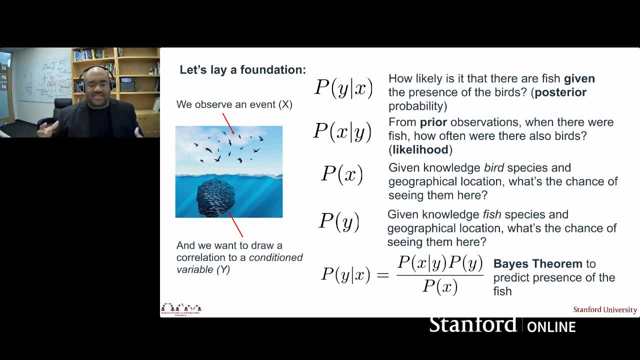 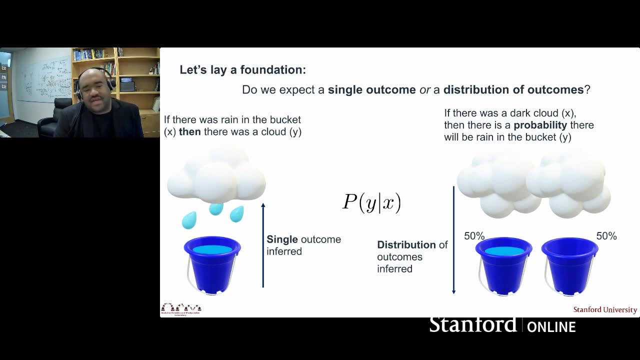 extremely powerful, as is statistics generally, because it's the art of effective guessing. Bayes' theorem is extremely powerful, as is statistics generally, because it's the art of effective guessing. Another quick intuition I want to give you here is this idea of: do we expect a single outcome? 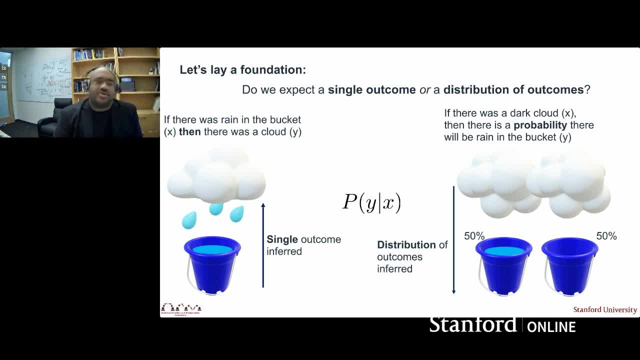 or potentially a distribution of outcomes. So here on the left-hand side, let's say, we had a bucket that was just sitting outside and the only way this could fill up is if there was potentially rain. So if there is water in the bucket, then we can assert that. 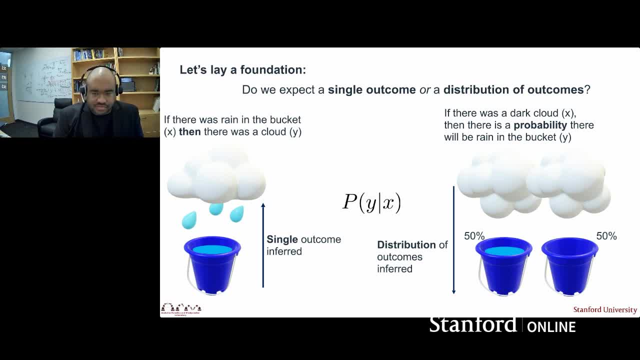 there was, at least, at some point, a cloud that filled it up. However, on the other side, if you look on the right-hand side of this image, if we see a dark cloud that potentially has rain, and I were to ask you what is the likelihood that this bucket is filled or not? Well, 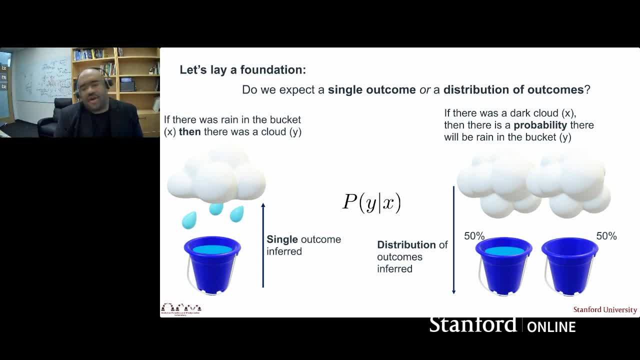 you have a 50-50 chance. Has it begun to rain or not to fill this bucket up? But given this cloud, statistically in the past you may have seen that this could have 50-50 percent led to some outcomes. So you have this distribution of outcomes versus a single outcome that 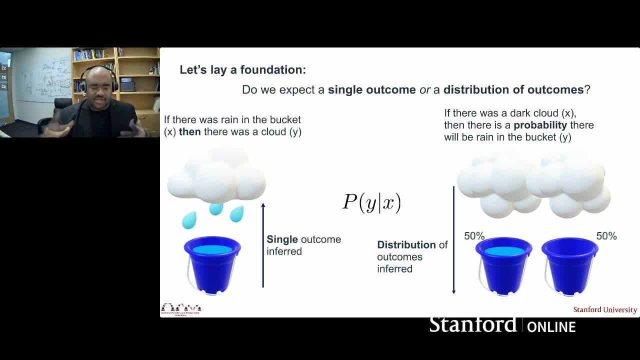 you can infer, And a lot of machine learning principles may rely on one versus other paradigms of thinking, depending on what you're trying to do. So perhaps you're trying to learn a relationship between variables where you say, if I had this outcome with this variable x, what is the? 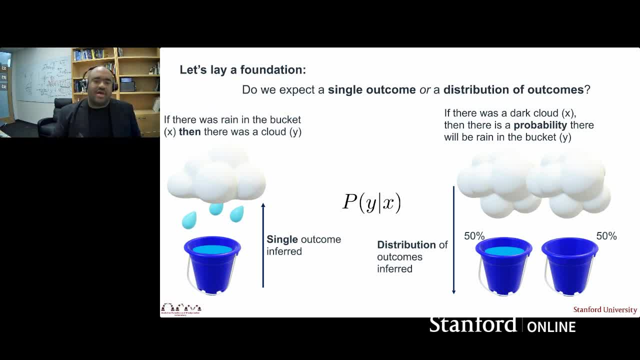 likelihood that this other thing happened. That's a regression model, But if I want to realize that could come out of this distribution, that's this more stochastic representation that I might want to capture, which you see here on the right, And both of those are useful, depending on your task. 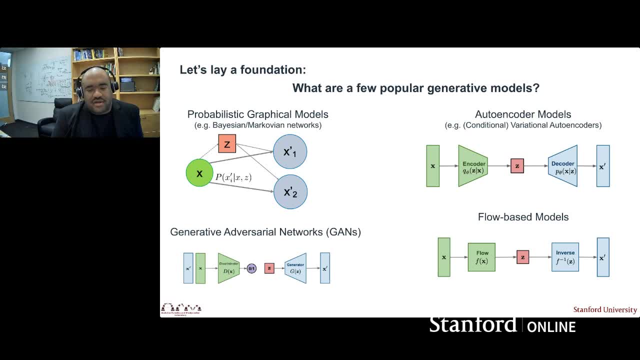 So to kind of again build an idea of the tools that are actually used to do this in the wild. I highlight these four types of models. One is a probabilistic graphical model, an autoencoder model, a generative adversarial network. 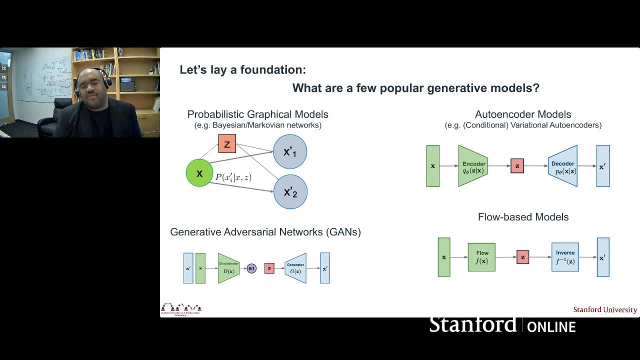 and flow-based models. The takeaway for these that I want you to have is there's this variable X, shown usually in green, here or blue, and then this variable Z, And what's happening here is this X is some observation of the world. 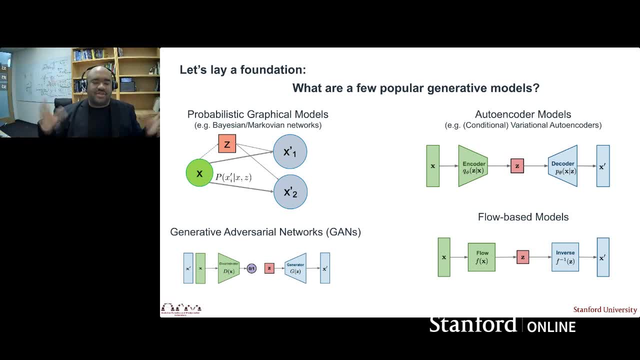 It could be a camera image or some other data- and you want your model to understand the key features of what that information, that information encodes, And you take an encoder model and you compress it to this what we call latent space or the code, and that's Z. 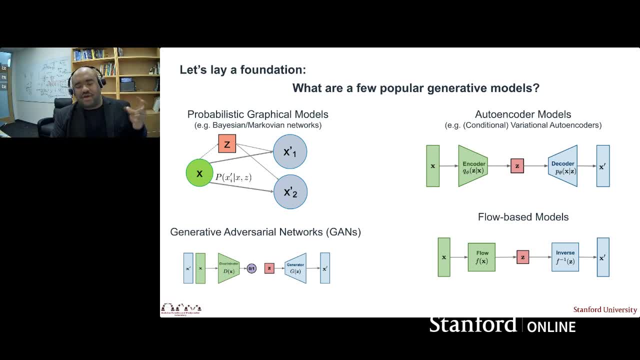 And this is an efficient way for the computer to think about some underlying relationship, And you use a decoder to then say: how do I go back to some representation of that state X prime where I've pulled out the key features to understand what was important. 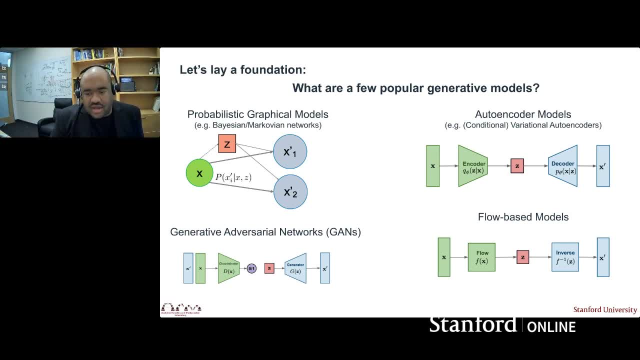 how do I perform salient feature extraction and so on, And here And so again it's saying: I'm given the raw data, I compress it to what's key and essential and then I can decompress it back to what was useful. 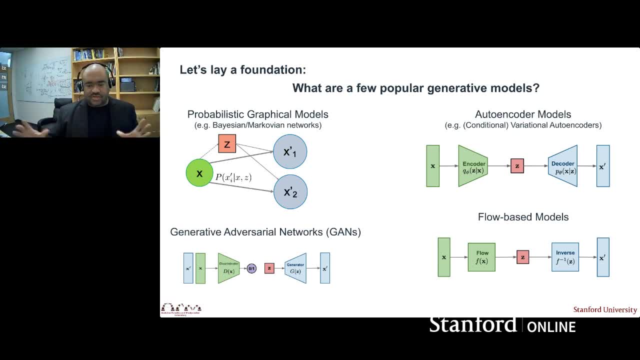 the big takeaways that I wanted to have, And so these are different ways to do it And we'll talk about some of these a little bit in more detail, but the goal is really to just give you again some knowledge of the jargon that's used in this space. 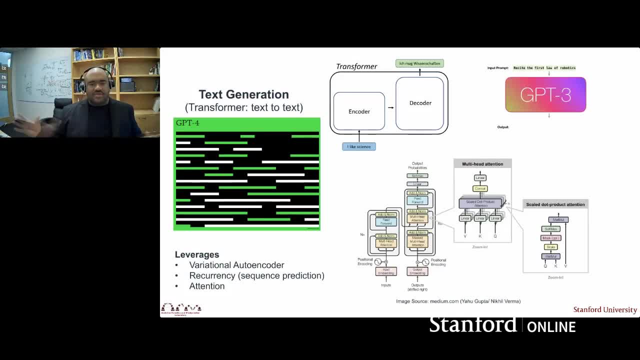 to accomplish these types of things. So what's under the hood? So the ChatGPT, which we all know and love, is using something called a transformer And, thinking back from that last page, there's three main components there that are going inside of it. 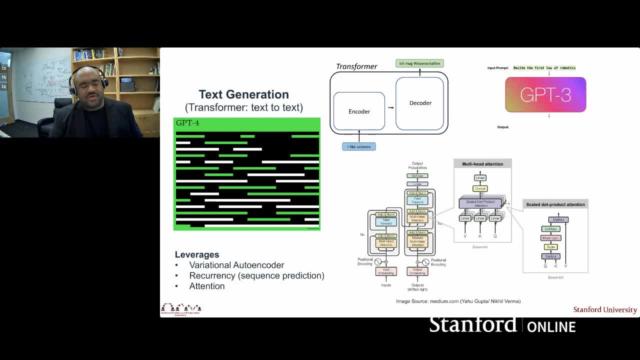 There's a variational encoder: recurrency, which is allowing you to perform a sequence prediction, and then attention, which is telling you what's the most important thing in the sequence of inputs that you should be paying attention to. So I first want to bring you 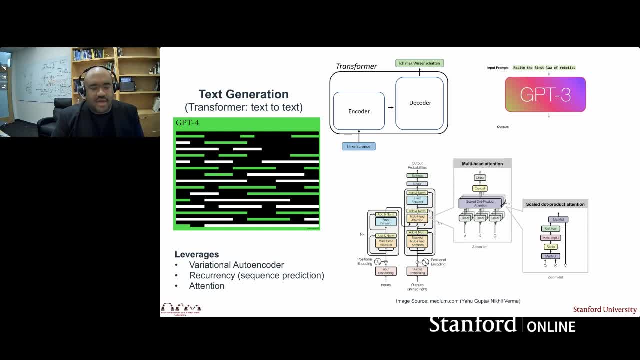 your attention to this middle image here. I like science and the goal is to transform this into German. So you have an encoder that is able to look over that sentence, compress it into a code and then, with a tag, output this translation in German. 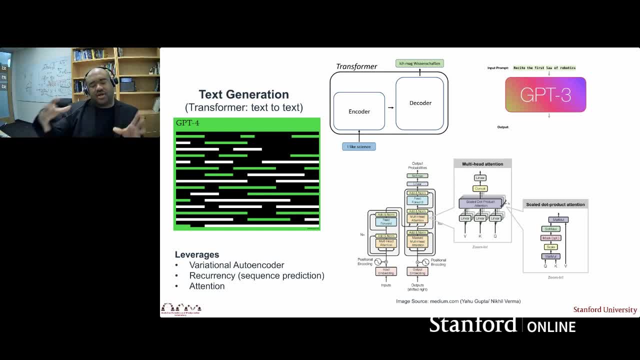 That's the sort of variational autoencoder structure coming into play. What's the most important piece here? How do I compress it And then output it into this other language where you would have the decoder related to, for instance, German or whatever other language you would want? 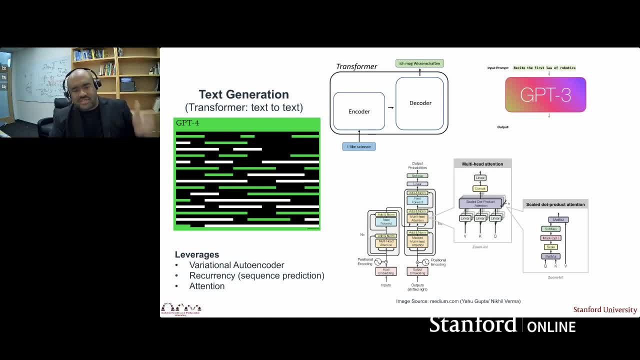 Recurrency says. you know what kind of sequence. how does the past words influence the future? So you know, the boy rode his bike to the park. is highly likely because of the fact that you had those words in front, The boy rode his bike to. 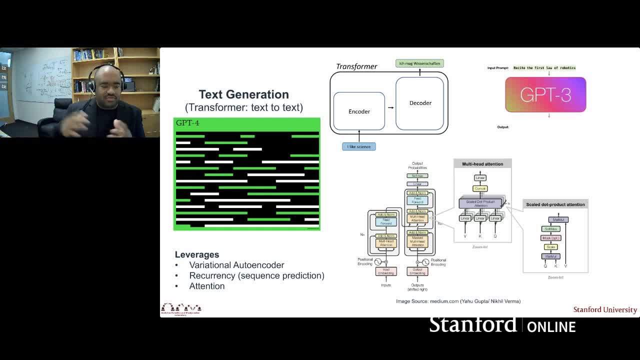 had high likelihood of a destination being an outcome. That's the recurrency. Attention means maybe not every word that you was spoken. The boy rode his bike. Maybe just boy rode and bike were the most important things you needed to actually infer what came next. 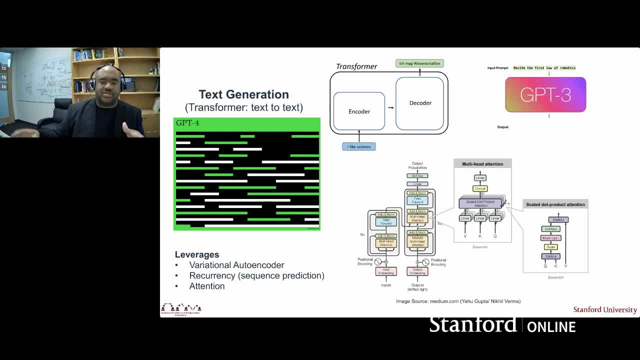 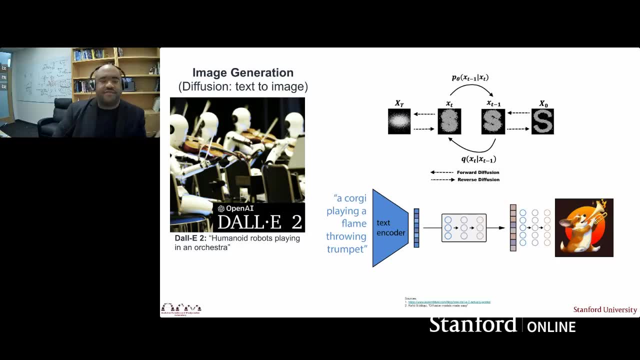 So attention says what are the most important things in the sequence I should pay attention to, to infer a particular outcome. Another is this idea of diffusion, And so it says I can have a relationship between a very crisp state. So here, shown in this middle right, X knot. 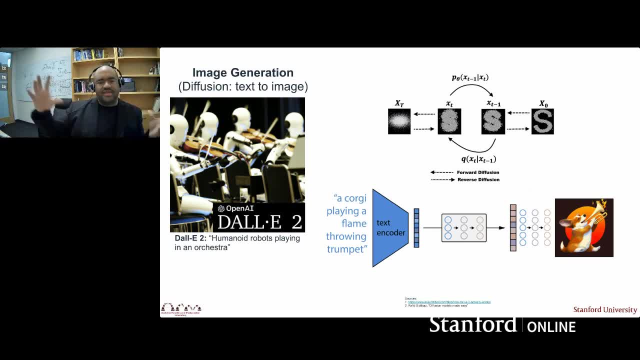 and this relationship of noise And the name of the game is to think about how I could make this noise, these variables that are positions that are random in position, how could I make them converge back to a salient state that actually makes sense? 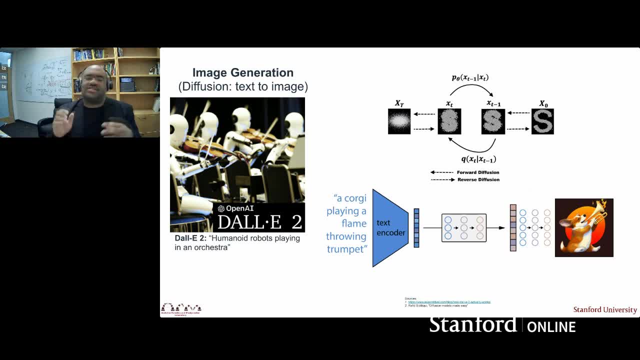 So here you see this noise condensing back to this S, And the name of the game here is: if you think of all of these points, think of them kind of like sand, If you had like a sand shaker, like sand shaker. 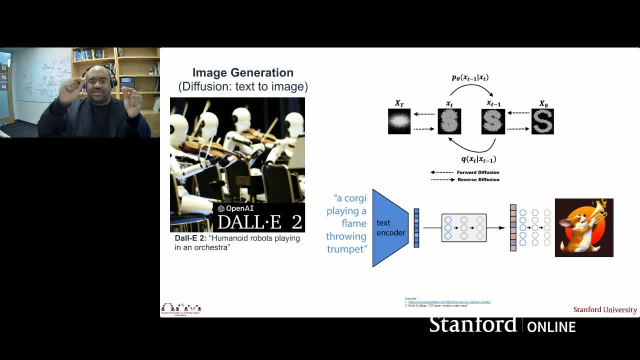 how would those sand shakers move back to their relative positions that would actually allow you to reconstruct an S. And so the modeling here says: how should every point move along that space, along the plane, to get back to its relative position on the S? 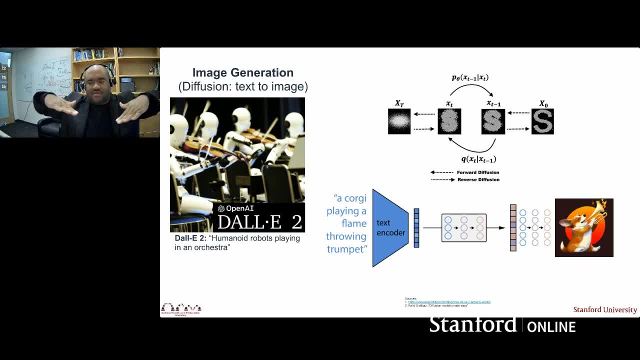 And whatever you condition on determines the shape of the ground. that would make that sand particle move back to its position in the S formation And that's what you condition on. So in this example for text to image, I say: produce me a group of robots playing the violin. 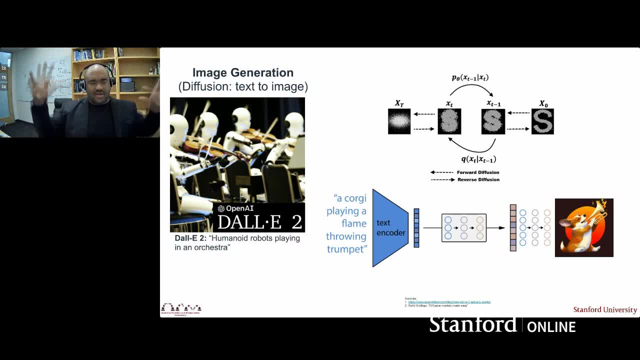 And then, given that, as a text input, it then determines how to take a noisy image and condense it back into a salient, realistic looking image that captures what you conditioned on, which was the text. And again there's this latent structure. 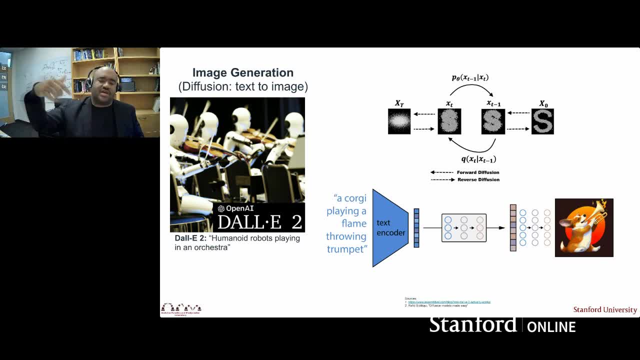 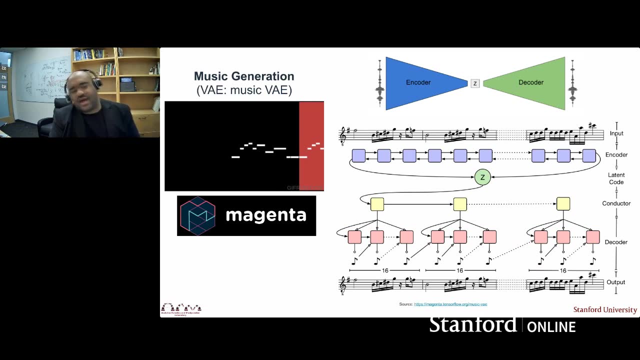 that's coming into play. that describes the gradient of how those noise particles should conform to give you back a salient image in this form. Another example here is music generation. So same idea I can put in a signal here, here, at the beginning notes of a song. 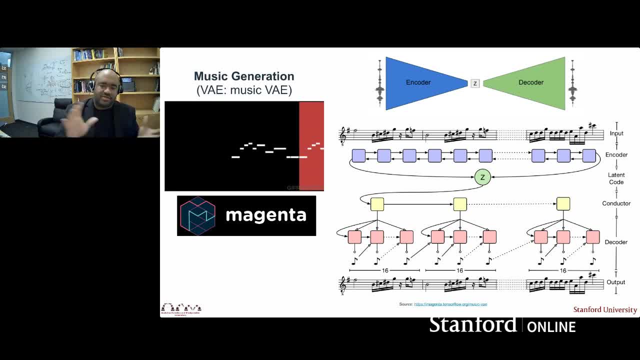 and then I can say, given all of the music I may have exposed this model to, what do you think should come next? And again, perhaps elements of features of this song are being pulled out to actually help you extract and reconstruct similar output music. 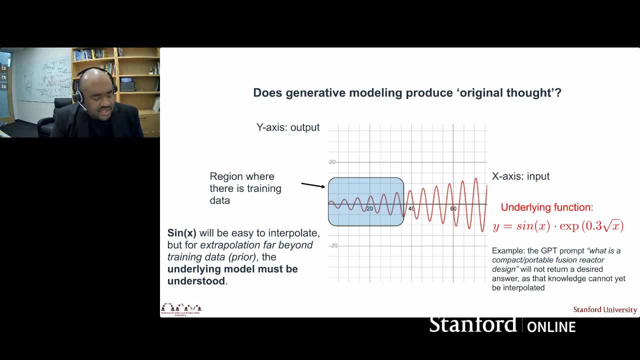 So, I think, a very important question here. we see these tools and we wonder how powerful are they. Is this the dawn of true machine intelligence? And I think these tools are very powerful, very useful, but I think, a very important thing we need to keep in mind. 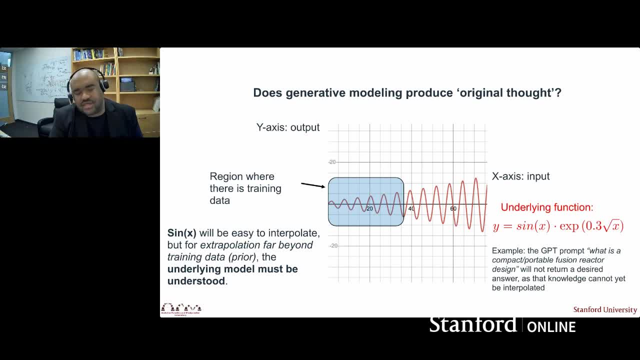 and what may actually, I think, still differentiate in some ways what humans are able to do versus robot, is this idea of original thought, And so I'll postulate this example to you, and then I'll make it more high level and intuitive as well. 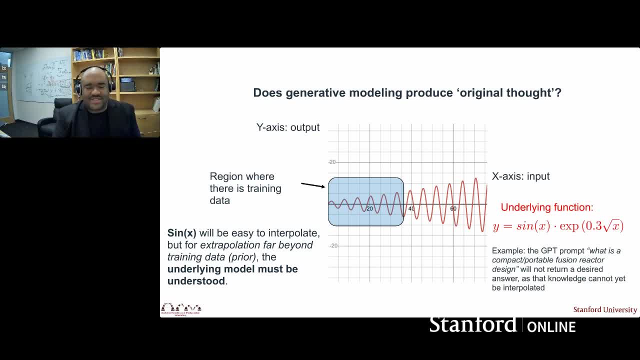 So again, please excuse the fact that everything's on the slide at once, but imagine I had a sine wave here. So X is your input, Y is the height of the wave and the blue region. you see, here it's the sine wave. 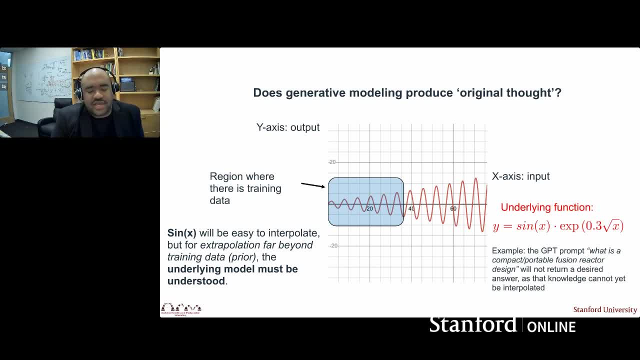 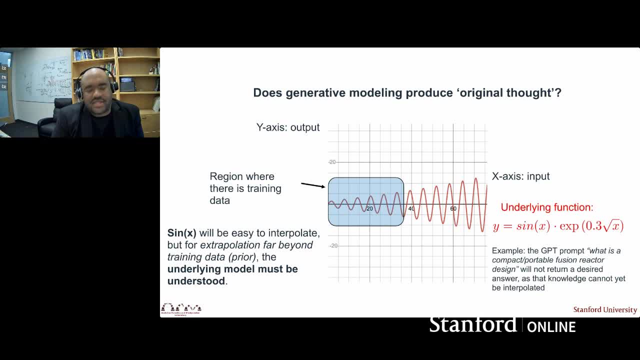 So over this span of 20 points the sine wave doesn't drastically increase in its magnitude. it's increasing fairly slowly. So it would be a perfectly fair assumption to assume in the blue region that all you would need to predict the Y is just sine of X. 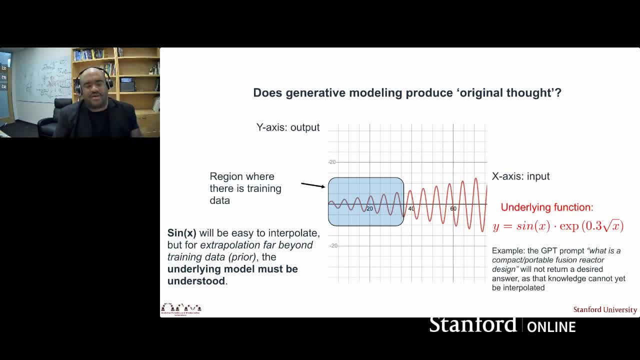 However clearly we can know with our external view here, However clearly we can know with our external view here, that that's not a complete view, that that's not a complete view of how this model would behave And in fact, it would be better. 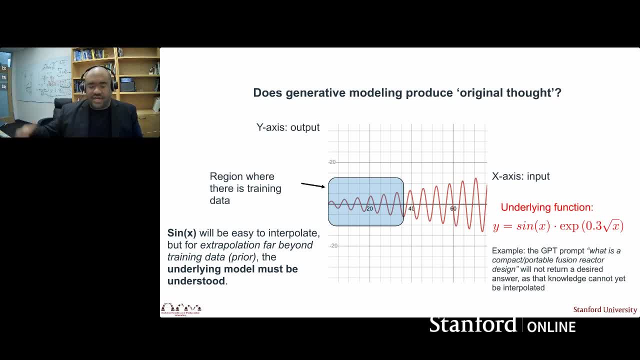 to actually be able to extract further, to have something that would predict points that are far outside of the region you were trained in, And so this is the challenge, right? How do you say if I expose my Chachaputee model to a bunch of verbal examples? 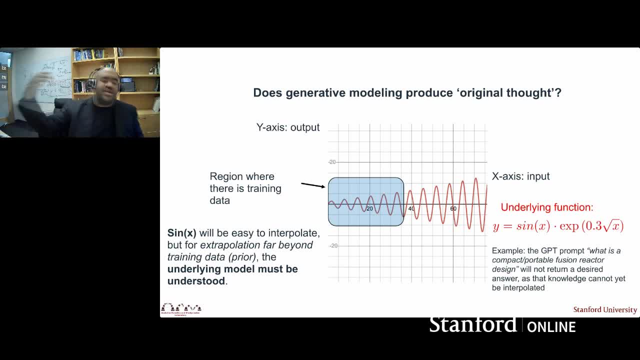 the internet as it exists today and I go create something new, and then I can say: and I go create something new, and then I can say: new, it can interpolate what currently exists. But if I say create something brand new, it won't. 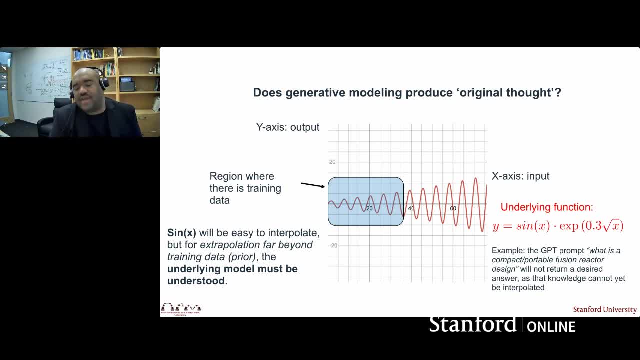 be able to do that. So the very easy example I put here in the bottom right is: if I ask my chat GPT prompt: you know what's a compact or portable fusion reactor design? It'll throw its hands up and say: I don't know. Now, does that mean that this is unknowable knowledge? I don't. 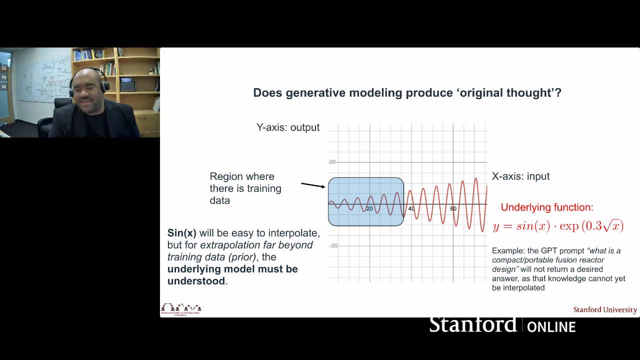 believe so We can look at, like Lawrence Livermore, and the advances that they have. I'm confident in the next few decades we will see a solution here. So if all of the knowledge to do this currently is existing or being built or could be built up by us, why can't chat GPT do this yet And it's 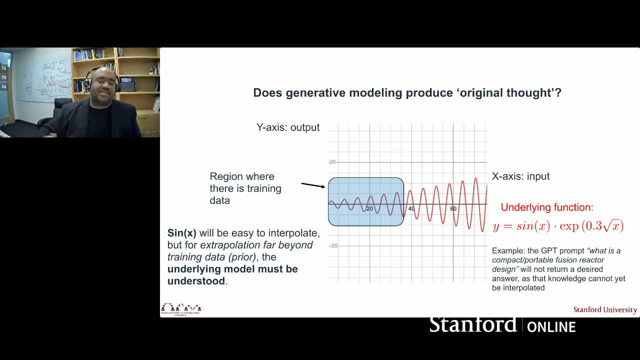 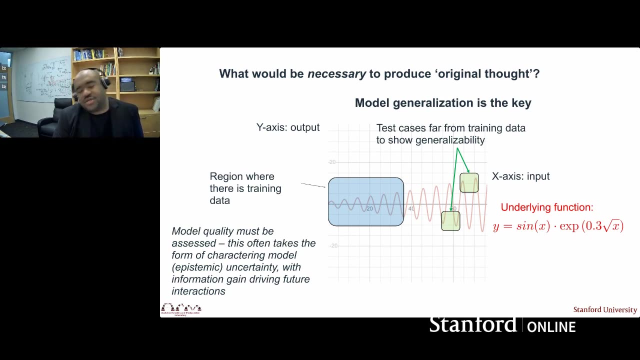 because it's interpolating from what currently exists and it's not extrapolating beyond the training set, beyond what it was exposed to. So how would we achieve that? What are some high-level thoughts that it would take to actually do that? Well, you know, to achieve this, you have to be somewhat self-aware and say: well, even in the 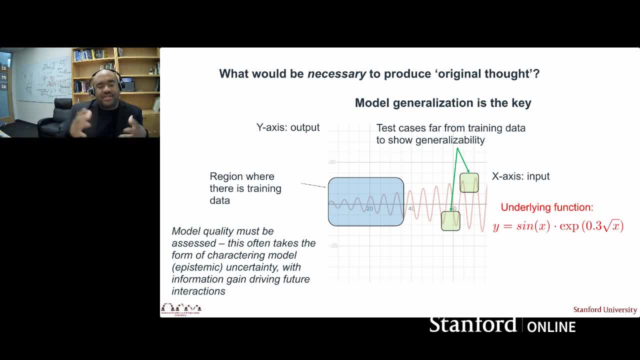 region that I'm exposed to. how do I make sure that I'm doing a really good job of explaining that behavior everywhere And maybe for some parts that are really far away? if I could gain access to those components, could I make my model actually perform correctly and predict those? 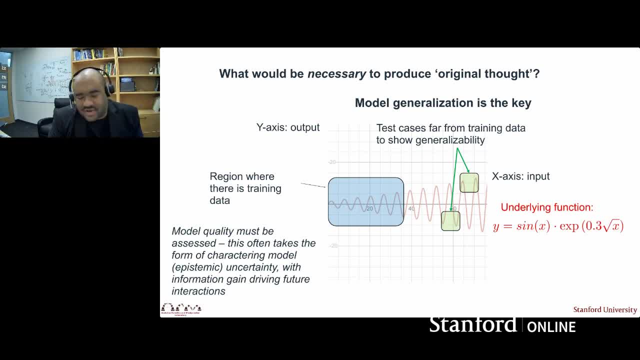 things that are very far away. I have a passion for physics, so I love to use this particular physics example- How even aspects that physicists are able to do to explain features very far away, like a few years ago, we were able to get our first picture of a black hole. It took the entire planet coming. 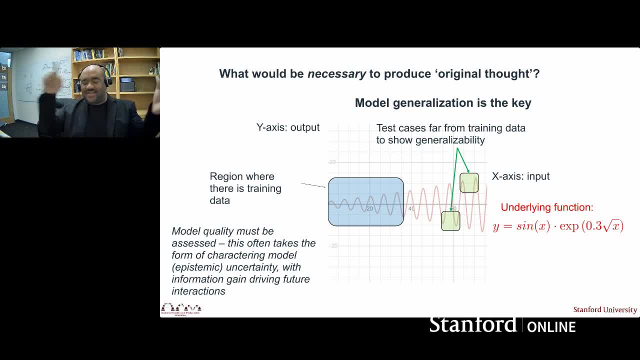 together to effectively create a camera that literally spanned the planet to get this picture of a black hole, And the equations that describe this were those that described things on a smaller and smaller level. So we go from Newton to Einstein to even smaller equations, And so you. 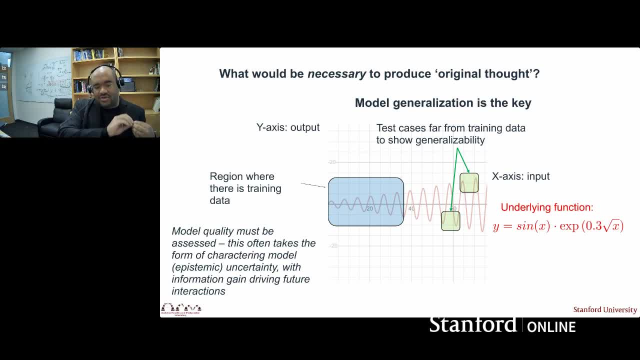 have equations that are more compact, that, as we understand our universe in a more fundamental way, actually extend and allow us to make predictions that are even further away, like a black hole. I use that as an analogy here. If I were to look at this sine function and I were to say, okay, I want. 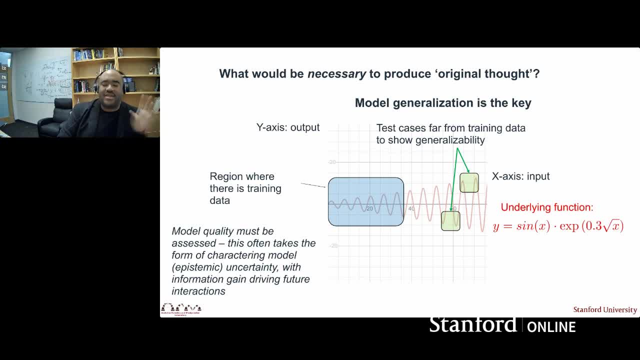 to have a description that is accurate everywhere. I need to be able to model the most compact form of this, of this equation, and have it be applicable, have it be accurate even far outside of domains, And so I believe the path forward for that is actually models that understand contextualization. 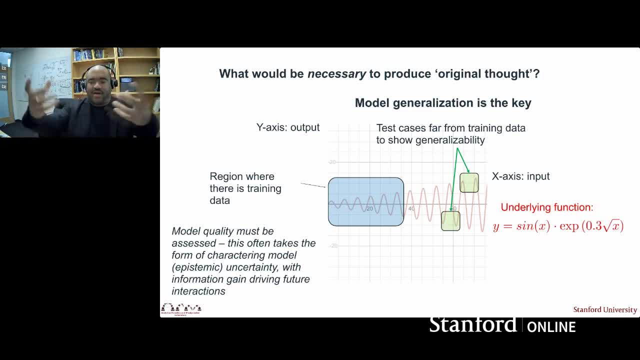 and are able to modularize their components and play them out and understand how they would affect each other, how they would behave even far outside of the domain they were originally exposed to, which is, I would argue, how we conceptualize things, We think about concepts, we form, 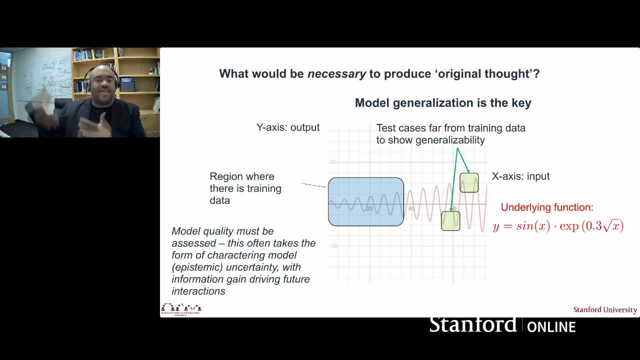 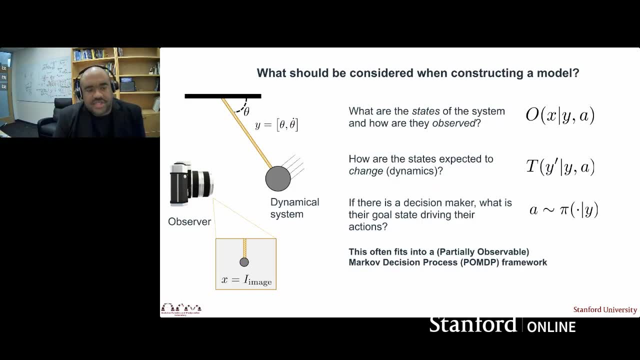 hypothesis by saying how these concepts should play together, and then we test them. That's the scientific process. So changing gears a little bit here. how should we, what should we consider when constructing a model? So here I've drawn a simple pendulum on a string. here where the pendulum has some mass. 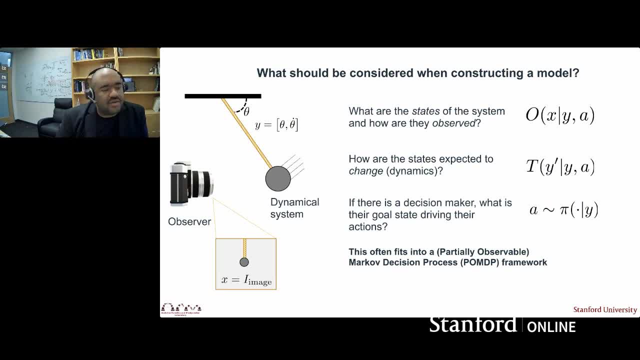 and it's moving back and forth. It makes some angle theta with the ceiling And you can think of the state. the most efficient way to represent the changing variables of this pendulum as the angle and the angular velocity, If I have a camera that's looking head on at this. 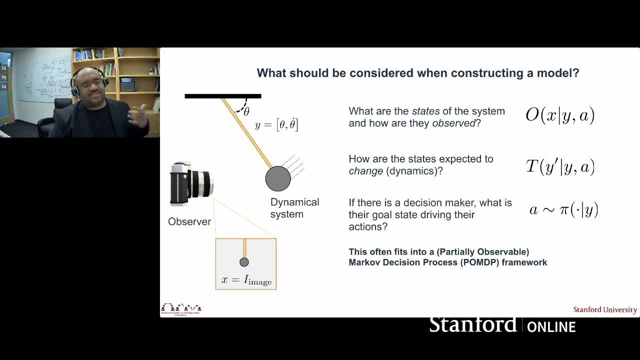 pendulum as it swings, I could try to extract the state from this image, And so the key relationships that I need to be aware of here include the observation. So if X is my image, this is what I'm observing, and I'm trying to predict and understand that relationship. I can. 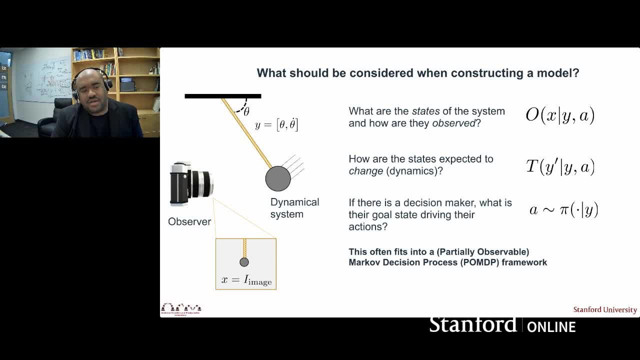 say, how is my image going to react to that? How is my image going to react to that? How is my image dependent on the current state, the theta, theta, dot. And if there's any actuation, if I have a motor or something that's forcing some motion, causing some action, how is my 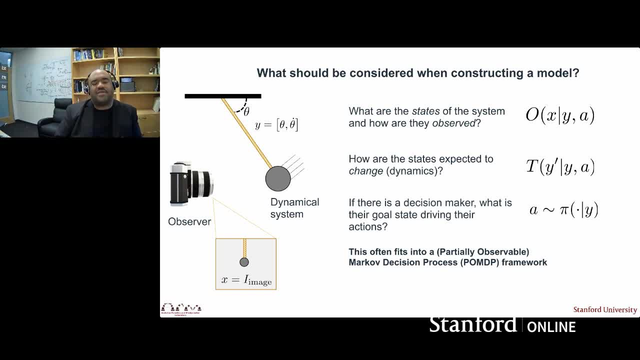 output image related to those variables. I can talk about the dynamics. How do things change? How do I expect the position and velocity of this pendulum to change, conditioned on the past position in any action that was taken? If there is a decision maker, 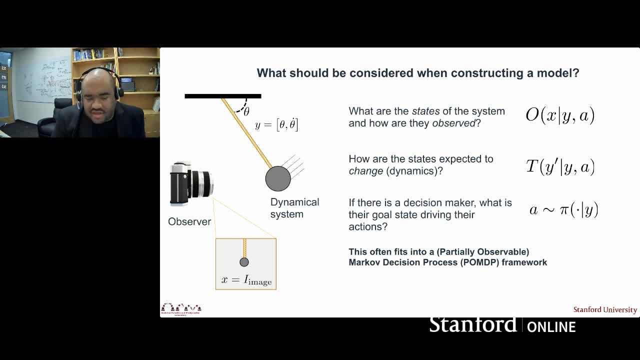 that's changing the state of my system, what's driving their actions, And this is, in the machine learning community, known as a policy in the analytical controls area. this is a controller description, And so I represent these in a probabilistic framework. 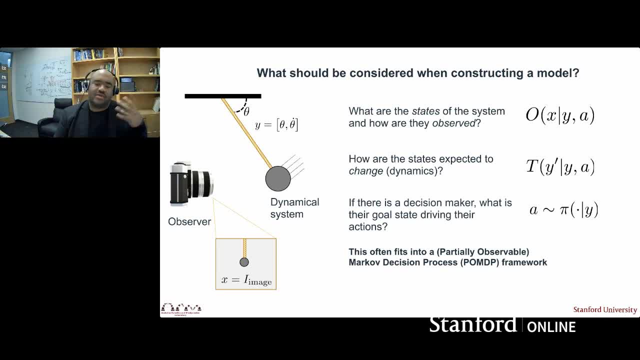 because it's a sort of catch-all framework, whether you're dealing with analytical equations or even different types of representations, And so this often falls into something called a Markov process or a partially observable Markov decision process, which describes how a state changes and 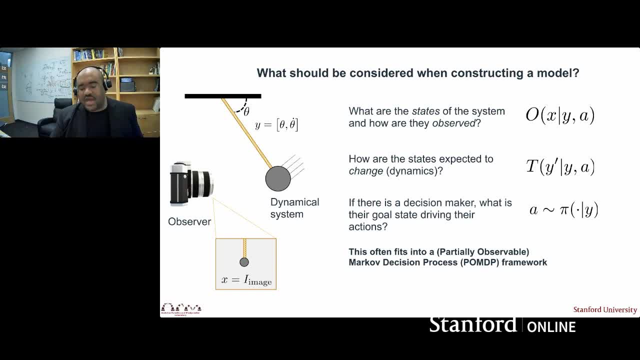 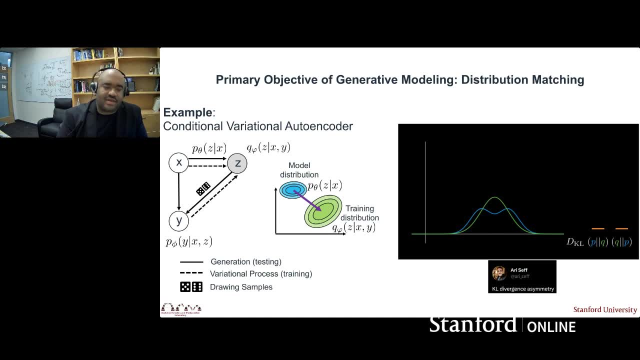 everything that may contribute to that change of state and how you might observe it. The other key thing here is when you begin to try and think about distributions of outcomes, you literally have a statistical representation here like a Gaussian. And so, if I have this shown in the middle, here some p of theta which represents my 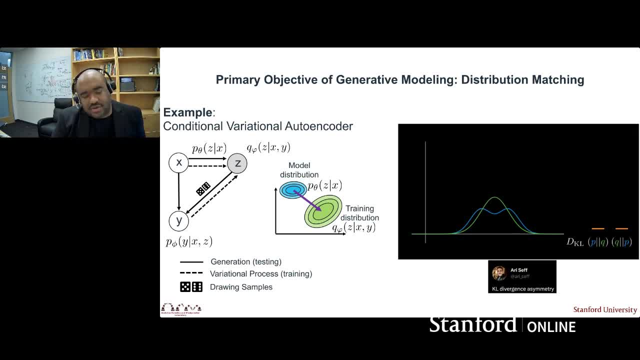 model's distribution and I had some training data that I exposed you to, which is this green q of psi. the goal is to match these distributions And again, let me ground this for you. Imagine I have a person that's driving around a track. 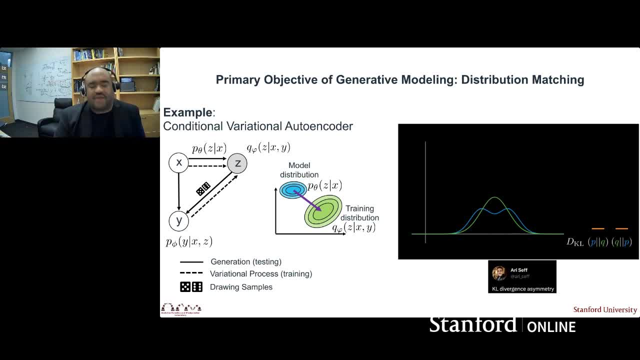 and I want to do a physical Turing test. I want you to, if you're in the stands, I want you to tell me if a person is driving that car, or if a machine is driving that car. How would you determine that? Well, perhaps if you watch the person. 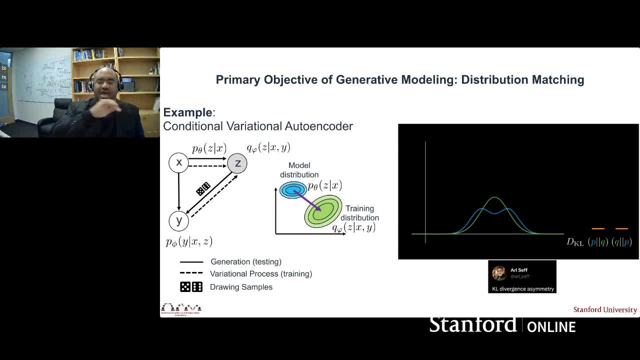 they're super efficient at this. they do some drifting, but you notice that their motion is not exactly perfect. While they're fast, the motion that they perform is not exactly perfect, Whereas perhaps if I showed you a machine driving around the track. 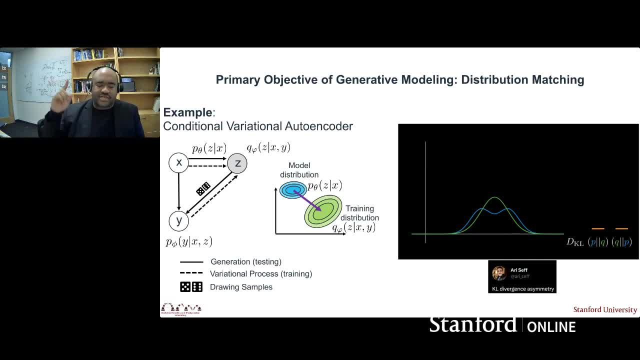 it would actually look like it was flying by a wire. Perfect execution every time, and that's how you would determine that a car or an autonomous vehicle was actually driving on that side. So if I wanted to fool you, the task I would have would be to add enough. 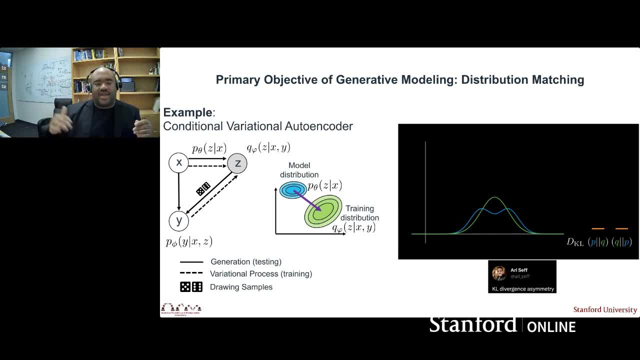 noise to the behavior of the car so that it would mimic that of a human, so you couldn't differentiate between the two, And so this is just an example showing how distribution itself can be useful for mimicking aspects of behavior. So with that I'd like to kind of move into more. 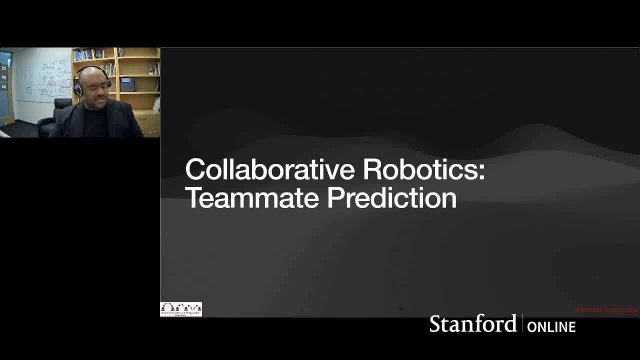 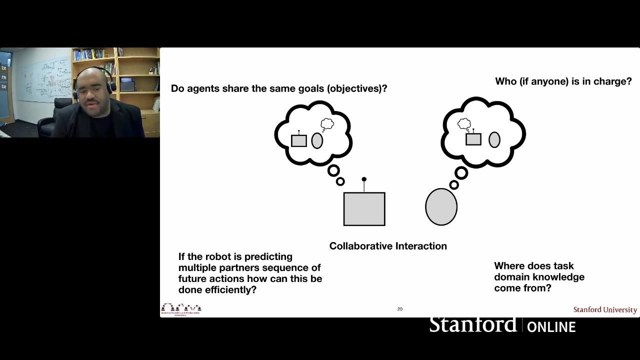 of this idea of team-made prediction and then tie this into some of the work that's currently being done in my research lab. So some questions we might have when you think about robots and humans working together is: how do they conceptualize each other? So here in this cartoon in the center, I've drawn this image. 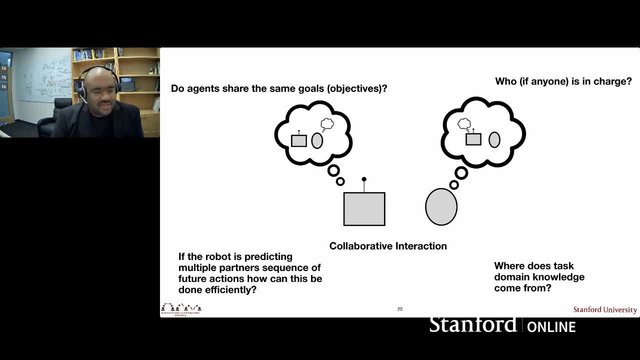 of a robot thinking about the team, and it even has a little thought cloud for the human. This is formally known in my field as a theory of mind of the first and second order. The first order says I just conceptualize myself and my teammate. Second order says I'm also trying to. 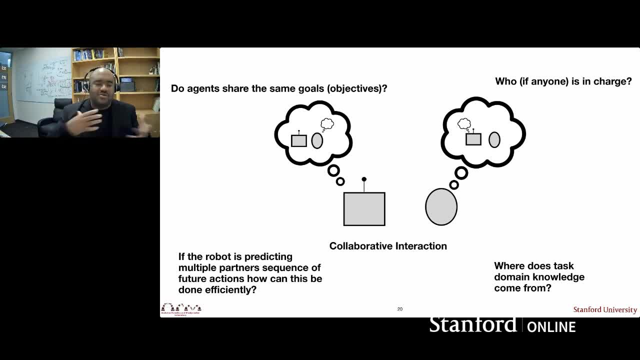 think about what my teammate is thinking about and use that to help me make decisions and plans. So here are four big questions you might ask yourself in this. First of all, how do I predict my teammates' actions in the space? Do agents share the same goals and objectives? Who, if anyone, is in charge in the team? 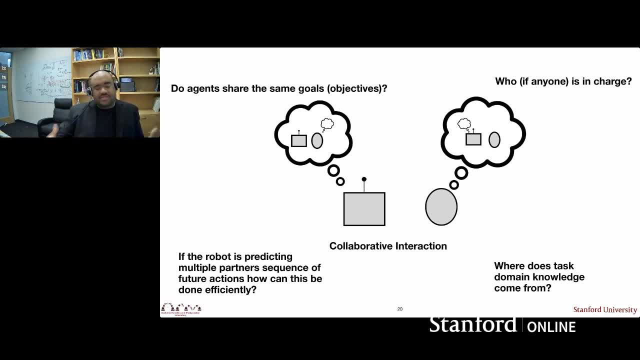 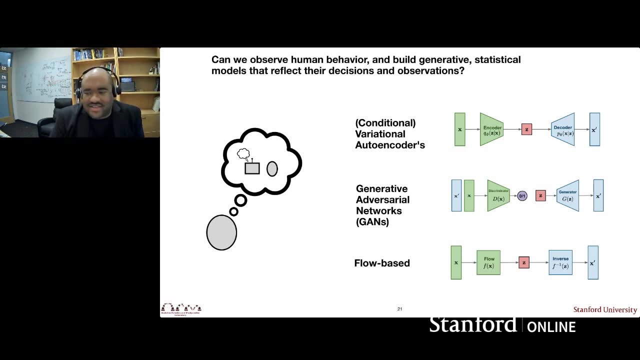 If the robot is predicting multiple partners and their future actions, how can this be done efficiently And where does task domain knowledge come from? Where did you learn to do the thing we're asking you to do? Again, our trusted tools come back to play. 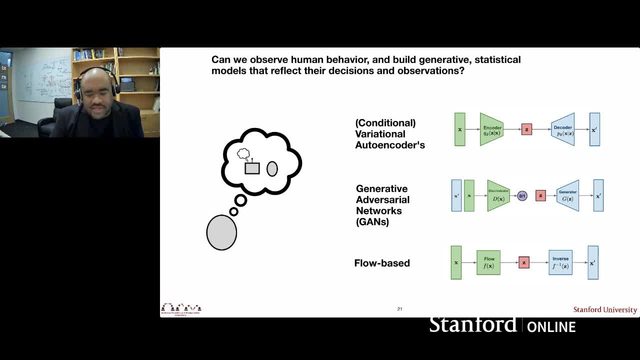 Autoencoder, generative adversarial networks, flow-based models- all of these can be useful tools, among others, but these are very popular right now. All of these can be very useful tools to try and infer and predict human behavior, given the exposure to their past behavior, as 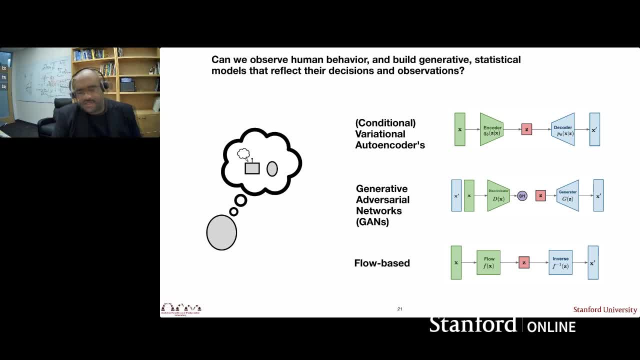 your training data. So I watch a human do something for some period of time, I collect these observations and then I'm trying to statistically match that distribution so that my robot can predict with some likelihood what might happen next, realizing that teammates are 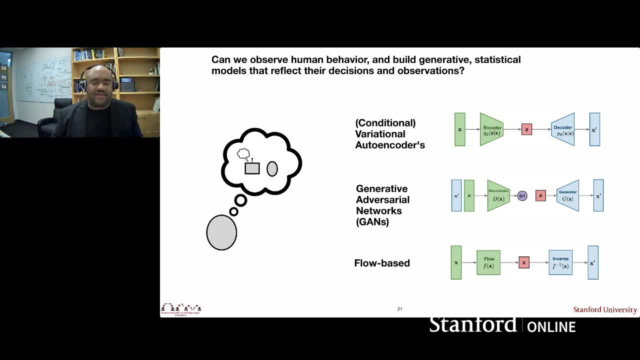 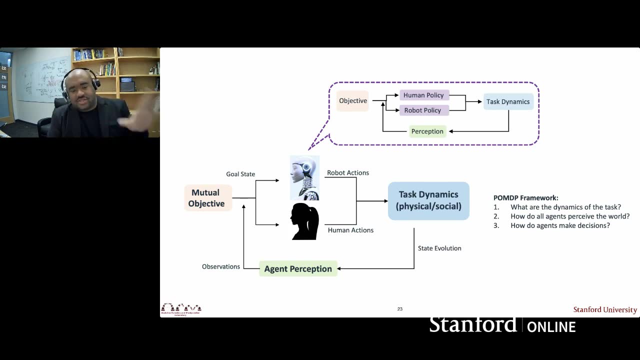 stochastic, So we don't expect to get perfectly right every time, but we want it to be very close within distribution of what the teammate might do. This provides a very nice description, too, of how this might work in a formal framework. So here you have this robot and human team. 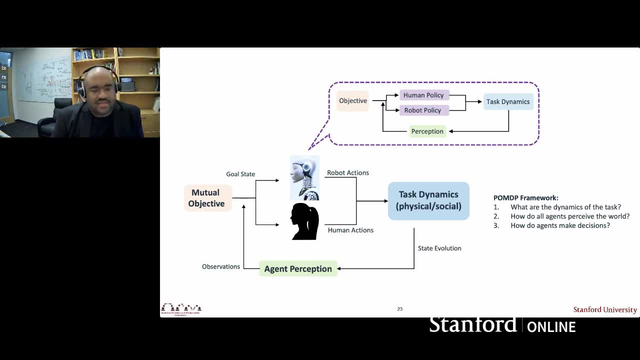 they share a mutual goal and objective. They both are able to take actions on the world or the task. This causes the task to change and we can measure this in terms of some sort of state evolution. The agents, human and robot, would observe that change and that would. 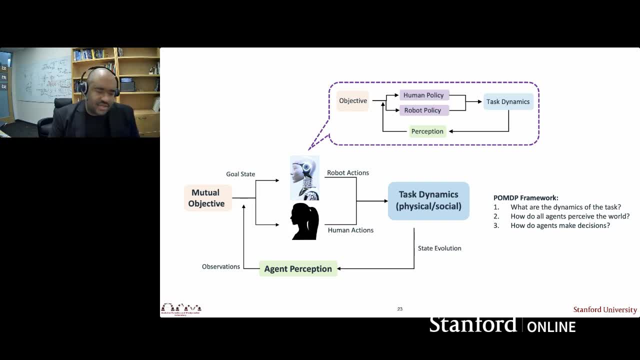 help them infer what future actions they should take. And we're postulating here that if the robot is able to conceptualize all of these components- the objective, the policies for both agents- how the task will evolve and how both agents will perceive the 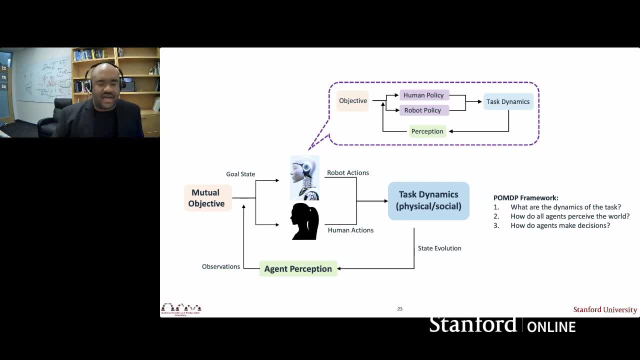 world. then the robot has a chance of rolling these things out in the future in its mind and saying: how does this maximize some measure of benefit or reward? And then I can then say: if I think of this stochastically, I could look at many different sequence of action pairs. 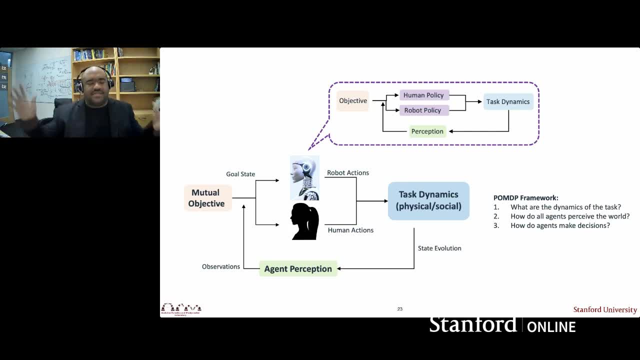 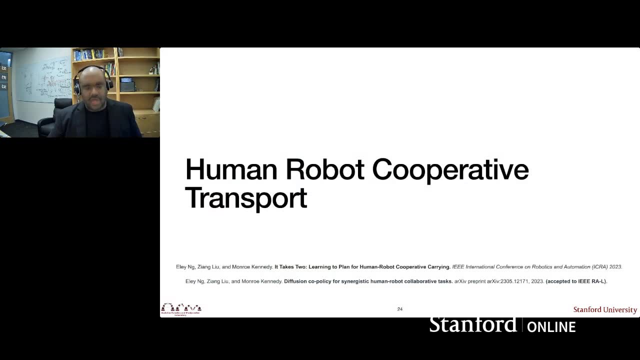 and then determine what action I should take next. that maximum, And so that maximizes some potential output, allowing me to be a better teammate with the human. So now I'll quickly show you a few examples in my lab that demonstrate this. I have a few videos. 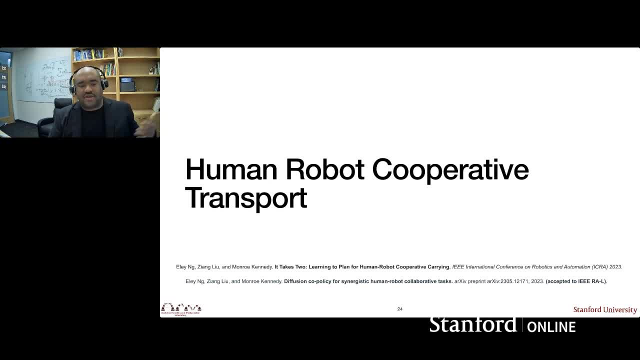 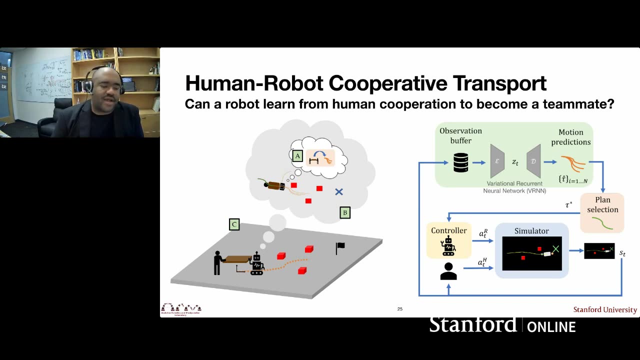 that won't play through these slides, but if you go to my website, armstanfordedu, under research, you can actually see some very cool videos for all the things that I'm telling you right now. So in this domain, one of the first things that I had was thinking about how a robot could substitute and serve as a 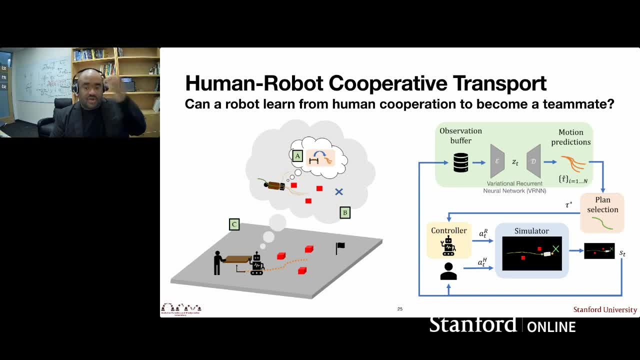 teammate alongside a human. So the concept is shown here on the left. So we have this robot that ultimately wants to help carry a table with the human, And what it does is in this sub-thought cloud. you see this A box it's able to observe. 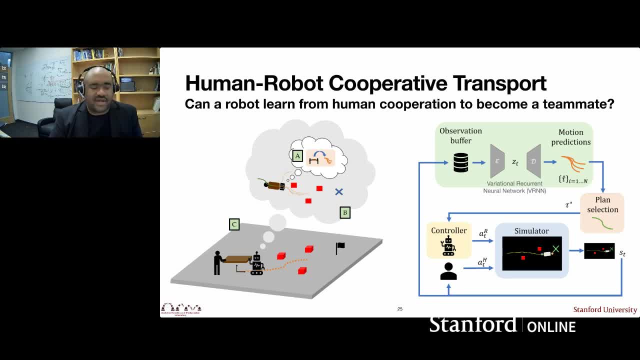 two humans work together, So we expose it to data where humans work together extensively. I'm in a very similar situation to what I saw two humans in- what would a human do? And it uses those statistical models we discussed to understand all of the possibilities that it was exposed to given a similar placement that it's experiencing. 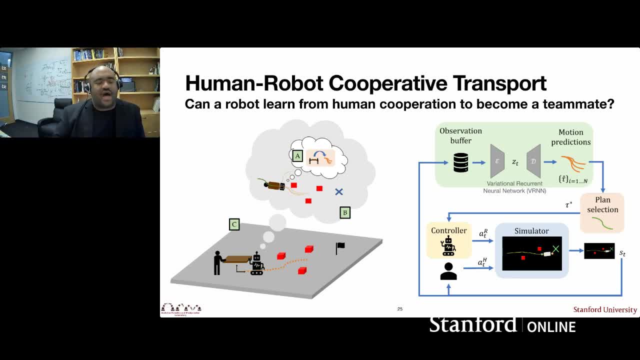 And after planning and looking at all of those potential outcomes in part C, it can say: this is going to be the outcome I'm going to pursue most, because I think it will maximize my reward of getting close to the goal quickly without striking one of these red obstacles. 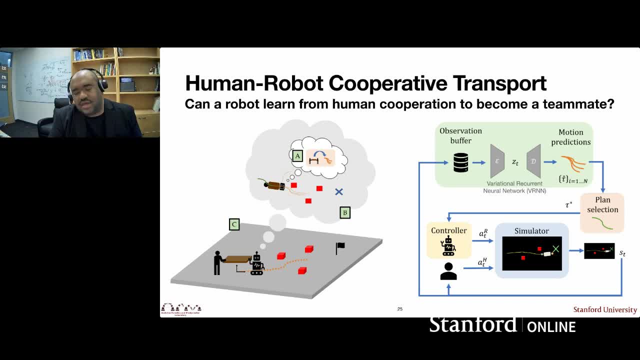 Shown here on the right is the methodology by which my graduate student, Ili Ng, achieved this. So here, the observation buffer is all of the human-human data that we collected where humans played this game together in a simulator. We then compress this into a variational, recurrent neural network, which outputs motion predictions, expected paths that are similar to what humans demonstrated for us. 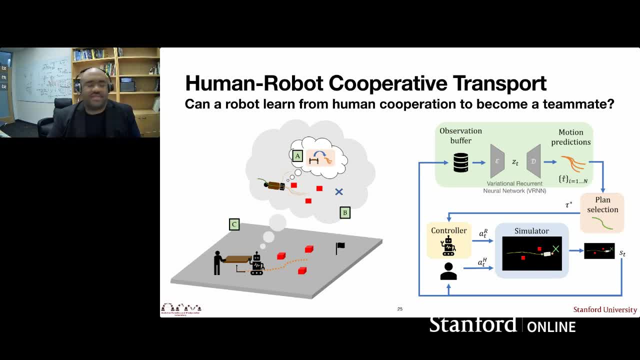 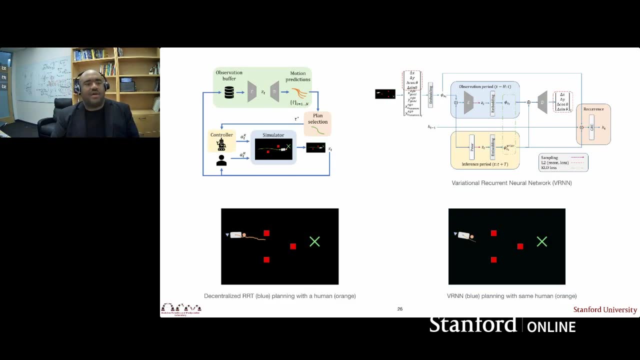 We then select what we believe To be the optimal path, given the distance traveled and other parameters, and then we tell our robot to execute that path alongside a human and we observe the outcome of that shared trajectory. And so we showed in our work that, if you compare this to RRT, which is a way of saying, let me just explore random paths and try to make sure none of those random paths I roll out don't hit any obstacles and eventually reach my goal, 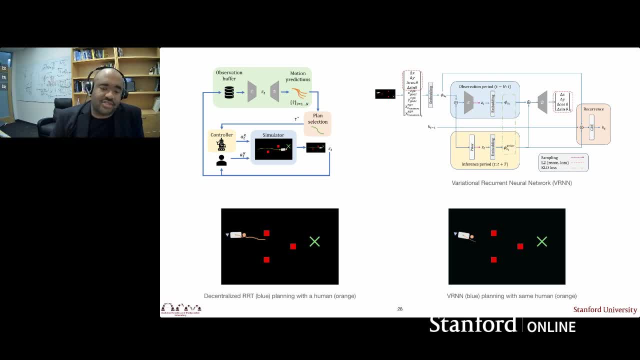 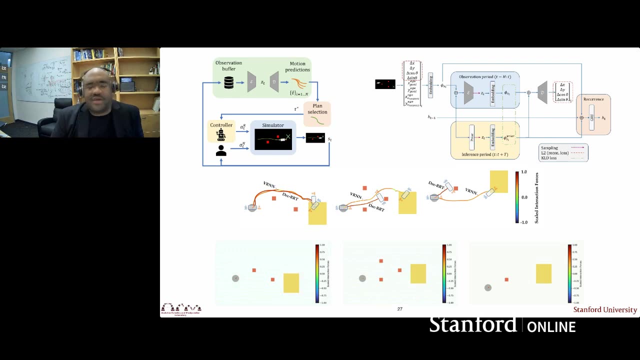 Compared to this method that's informed by what humans demonstrated for you, we're able to show that the VRNN, our method, actually produces much smoother outcome paths in the end. Additionally, you might say when you're doing this task, maybe you followed an efficient path, but how do you know necessarily that they were more collaborative than if they were to pick random paths that didn't necessarily hit an obstacle? This is an example of a more advanced method that we're able to use to explore random paths and actually reach our goal, And so we're able to show that if you follow an efficient path, maybe you followed an efficient path, but how do you know, necessarily, that they were more collaborative than if they were to pick random paths that didn't necessarily hit an obstacle? 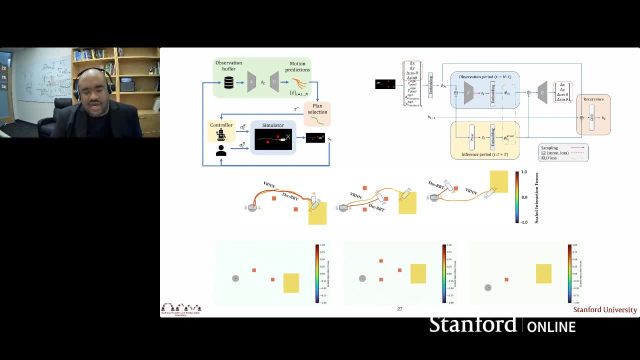 One way to think about this is through something called interaction forces. And so if you were playing tug of war, tug of war is literally a game of inducing stress in a rope because there's disagreement. One team wants to pull the rope to one side. 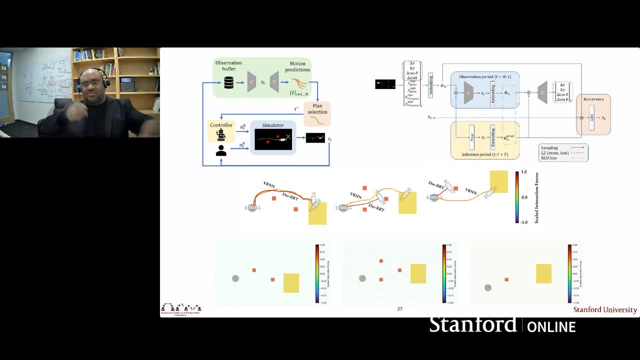 The other wants to pull the team to the rope, to the other side. There's these really large tension forces inside of a rope in the game of tug of war. However, if I were to pick up an object in my hand, perhaps I'm applying some forces just to localize it. 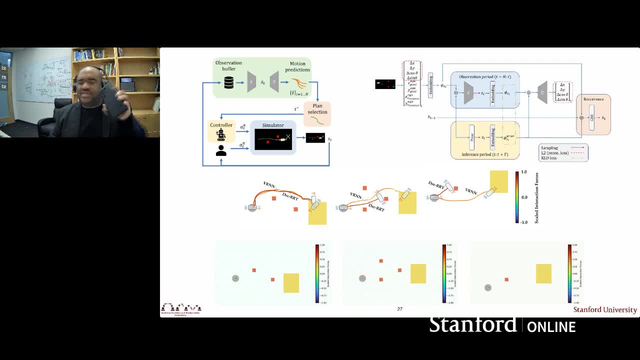 forces just to localize it. but i might not be squeezing this with all of my strength because there's agreement between my fingers on how i actually want to move this object. so one measure that the field has agreed upon is this notion of interaction forces. how much stress. 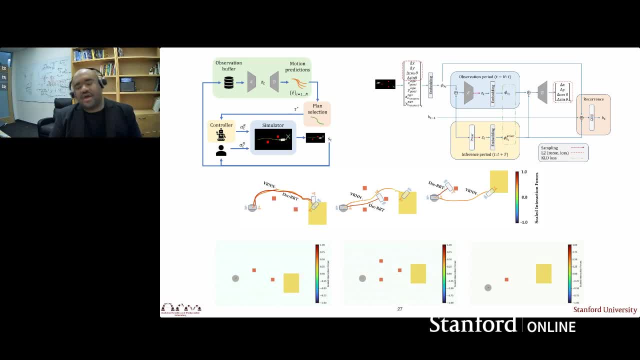 or compression are you applying to the object you're carrying, and how can that be used as a measure to measure consensus between the agents involved? and so what you see is, if you have two humans carrying something together, the interaction forces are low. they're not zero, but they're low. 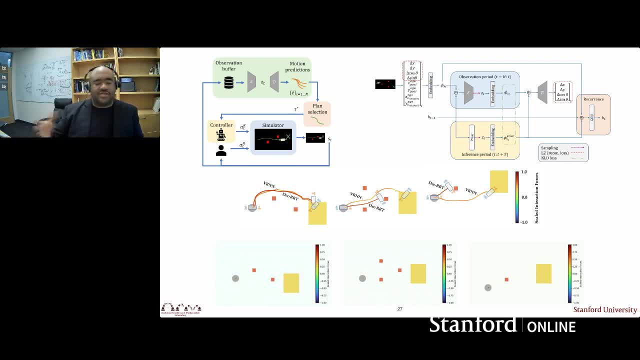 and if you use our vrn, they're also pretty low. if you don't and you use the sort of random path planner that shouldn't collide, you'll see that these interaction forces, the tug of war, is quite high. it was hard for the robot and human to reach consensus. 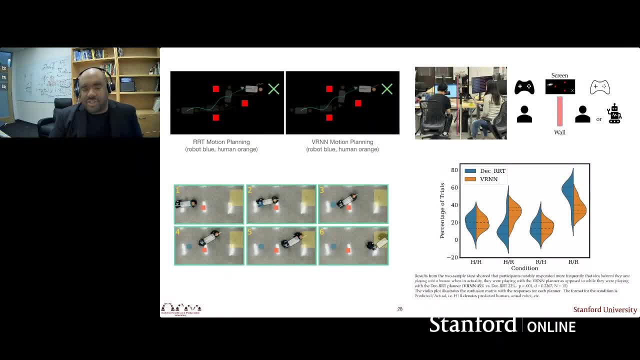 another really cool aspect here is this notion of the turian test. so we did this experiment where we said, okay, we're going to set up a barrier and we're going to have a participant work with this simulated partner in the carrying task and we're going to have them do a bunch of trials and in some of them they're going to 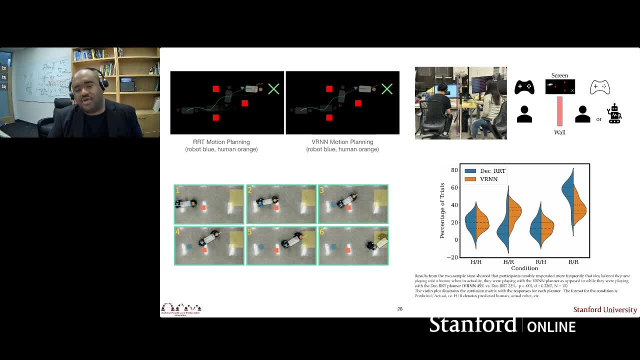 be working with a robot and others are going to be working with a human, and we want to know if they're able to correctly identify who they're working with based on the behavior that they experienced as they played the game, and so what you see here on the bottom is a number of human. 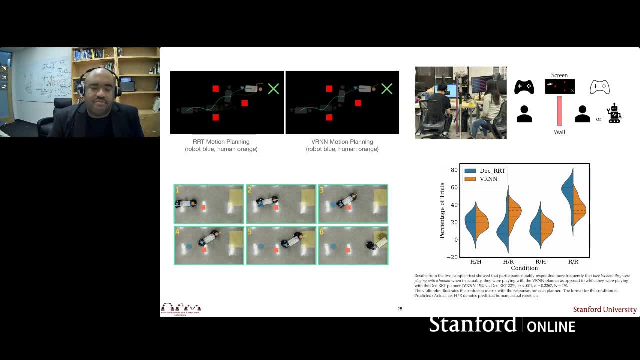 experiments and what we see on the bottom right are the results from that experiment. experiment blue is the sort of random path generator which we don't expect to succeed very well, and vrnn was our method that was informed by watching humans work together and this x-axis. 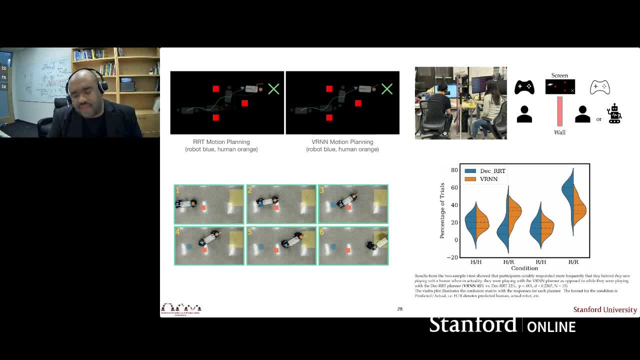 gives you what the human thought versus what it actually was. so if they thought it was a human- and it was a human- they got that correct. if they thought it was a robot r, given that it was a robot, What we saw was, with our method, we actually did a decent job of confusing people when 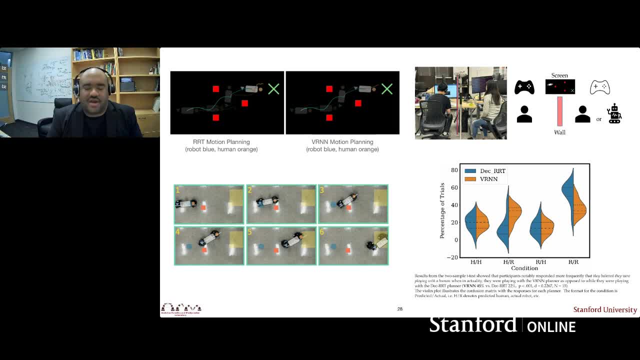 we actually had the VRNN system And this is just a violin plot. so this says all the data that we took. what's the distribution of that? in case it wasn't unimodal and you'd like to see the true distribution? 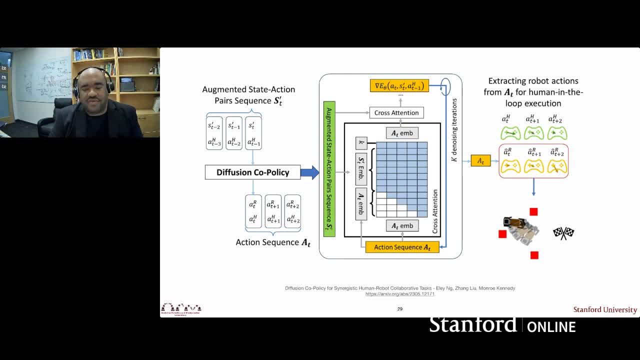 My student extended this work and I encourage you to again check out her really cool video where we actually said: now what if we used an even more advanced method to capture and model behavior? So for that we used a diffusion co-policy. 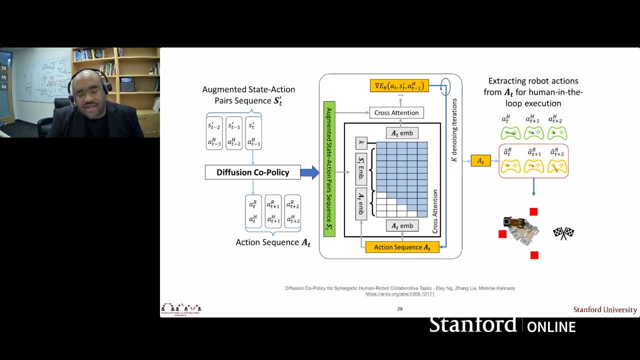 And it turns out that when we expose this diffusion co-policy to examples of human data and then we transported that to the robot, the robot began to exhibit very interesting high-level behaviors. In particular, some that you'll see in her video includes the ability to serve. 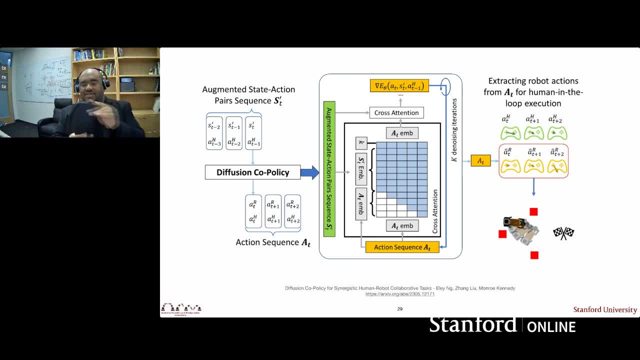 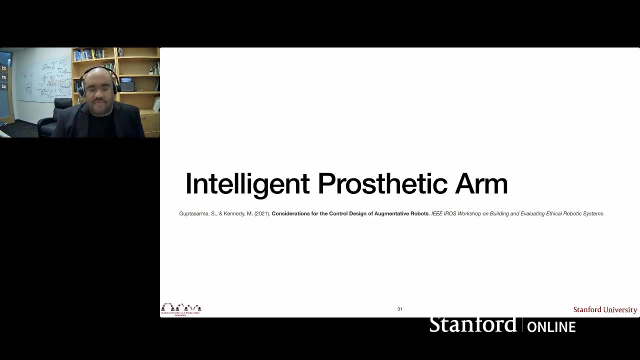 as a leader and then transition to a pivot, to then become a follower, so that the table could efficiently navigate the obstacles. And when we saw that, that made us very excited. Another project I'll quickly mention in this space uses the same type of tools, but applies 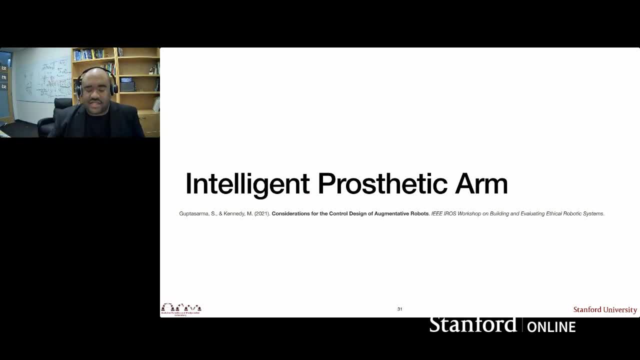 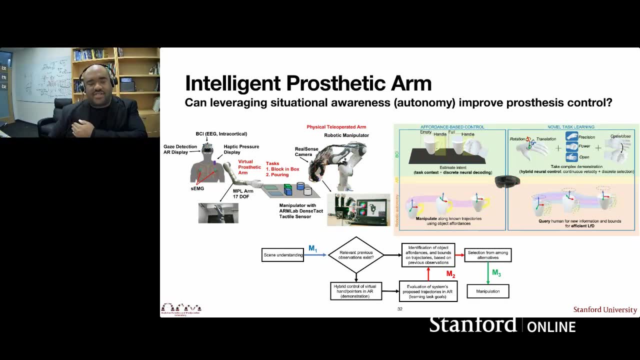 it to a completely different domain, And that's the intelligent prosthetic arm. So in this instance, imagine, someone has had a shoulder disarticulation, So they don't have their entire arm, And we want to endow them with either a prosthetic arm or a tele-operated arm so that they can. 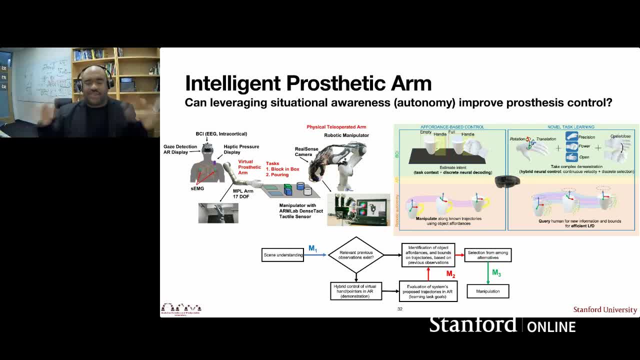 do complex manipulation tasks. again, There's two ways to think about this. One where you say, well, we know all the tasks they might want to do, like drinking from cups, picking up a fork, And then there could be an instance where you need to teach them how to do a novel thing. 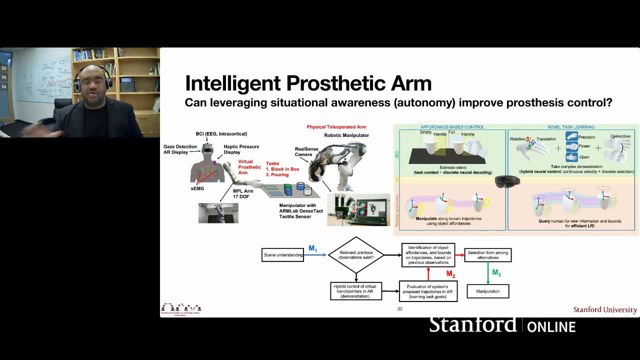 How do I teach you how to move the hand in order to complete a task? And it turns out that this same type of framework Where you say, given the tasks that are there, how do I extract their intent from their gaze? If I have them wearing a headset, what are they looking at? 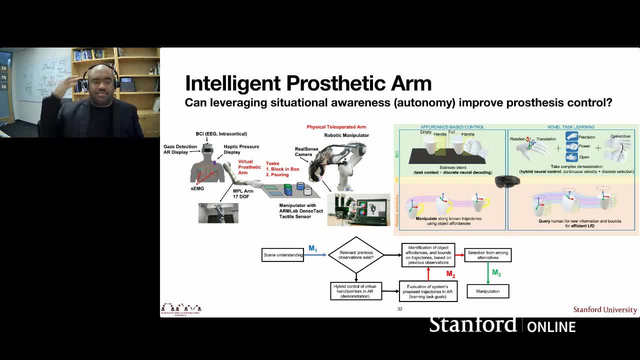 I could use EEG intracortical to understand their brain waves how. that might give me an idea of what they want to engage with Their EMG, so any muscle actuation they're able to provide. How can I condition on all of these inputs, be them limited in order to control a high? 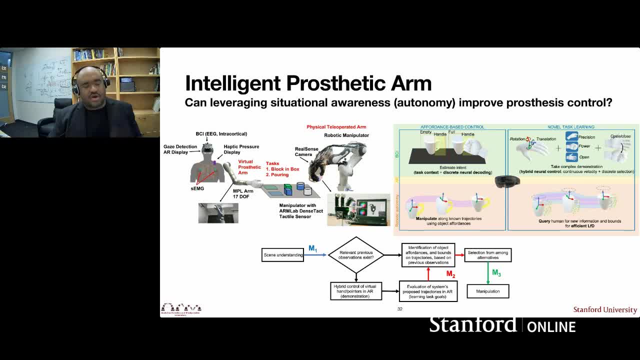 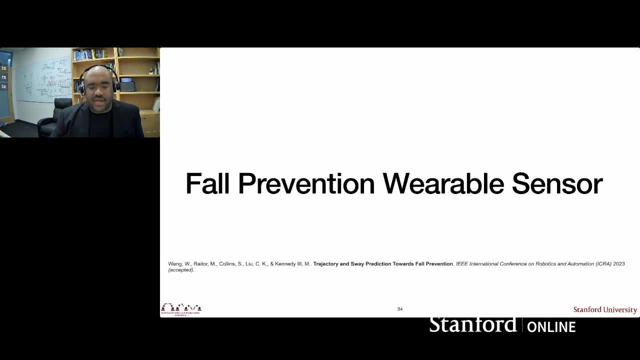 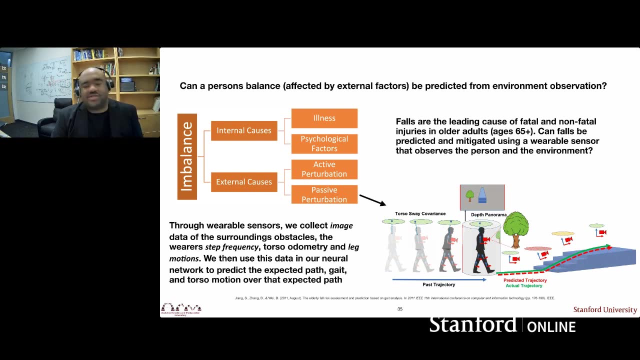 degree of freedom, Right Yeah, So that's one way to think about it. Another I'll mention to you is this fall prevention wearable sensor. So in this domain, we think about particularly what might lead to imbalance in a person, And it turns out that this is actually a leading cause of fatal and non-fatal injuries in older. 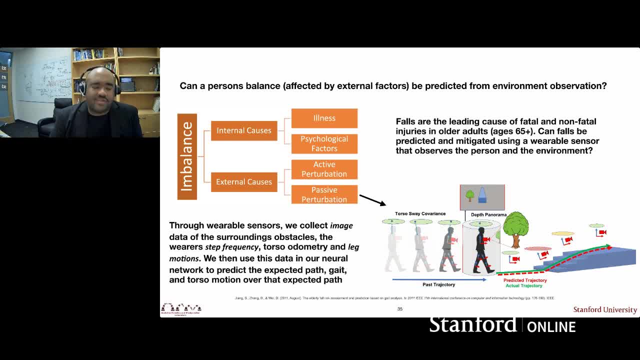 adults, Those who are 65 and older, And the question we had is realizing that falls can be caused by internal things like illness and psychological factors, But they can also be caused by external things. So if they bump into something or something bumps into them, we're saying: well, what? 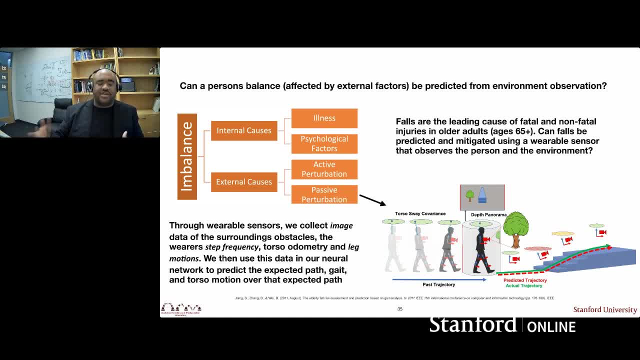 we can do right now is think about those external factors and particularly how they're walking in an environment. So a passive perturbation. You're tripping over some steps, You're bumping into a wall or something Can we understand, given how you've walked and watching a whole bunch of people walk? 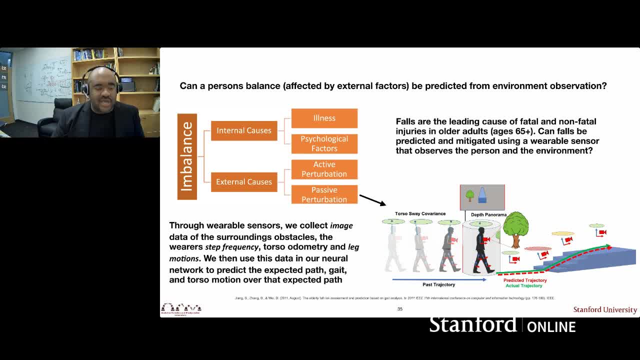 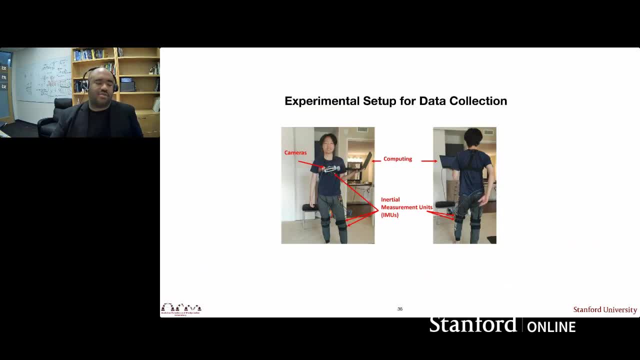 can we predict how there are features in your environment that might potentially lead to imbalance? Yeah, Yeah, Yeah. And so my student. he made this initial wearable sensor that includes a camera that's mounted on your torso, IMU's that are located on your legs. 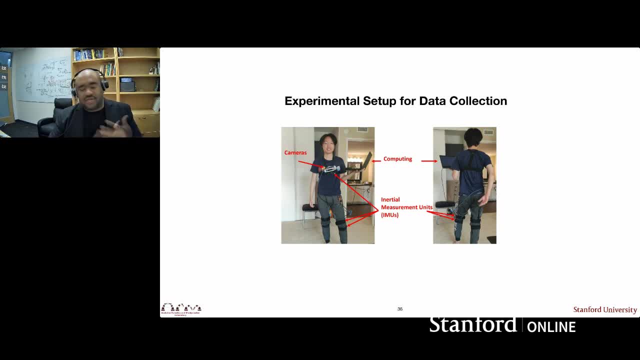 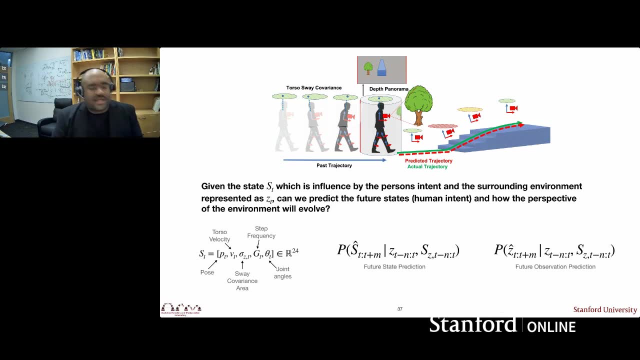 And the idea here is that, using these, he can observe the environment in order to use a machine learning model to accomplish this. So now we're back to our problem statement, And while we'll use some fancy models to accomplish this, it's very useful to formally say what 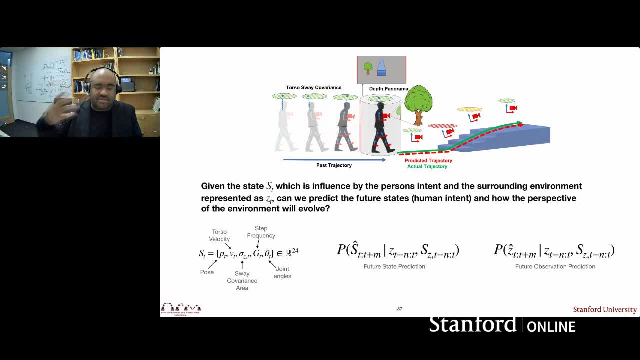 our state is, we can represent our objectives in a probabilistic manner. So here our state includes: what's the pose of the person, Where are they in space, What's the velocity of their torso? If their motion of their torso, if they have some natural sway and cadence, can we actually predict that sway, that cadence? 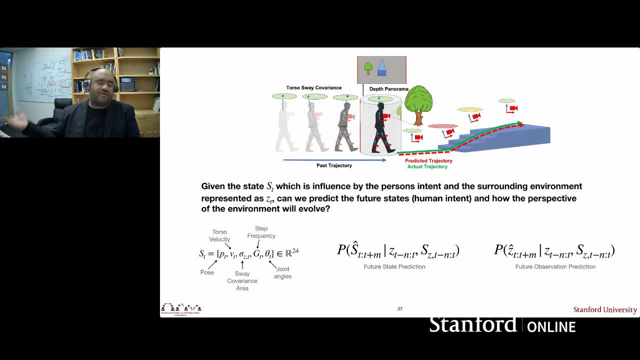 and then monitor that change in case that might inform us about potential imbalance? Can we watch their step frequency and the joint angles in their legs? And so these two probabilistic statements says: given how they've walked so far and the environment, can we predict? 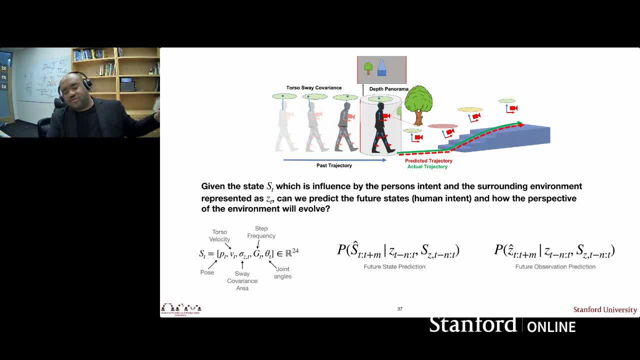 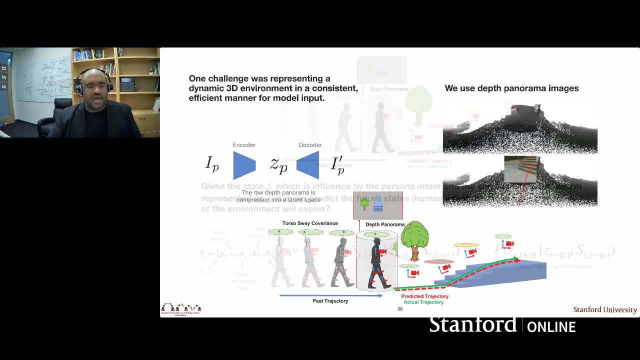 where you're going to walk in the future And, given what we've seen so far and where you've walked, can we predict how the environment will change around you? So the first challenge we had for this was how to represent the environment in a way that a neural network could digest and use. 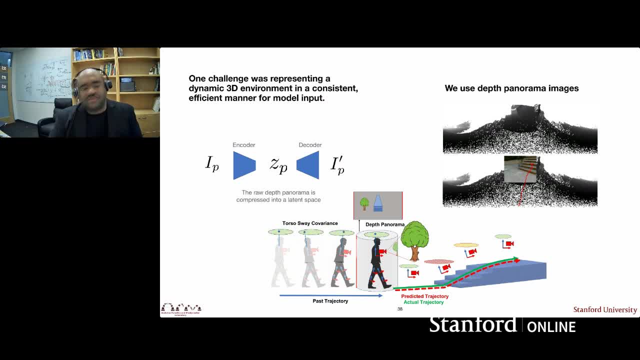 for prediction. So for our first step, for that, we used this sensor that was mounted on the torso to collect data. And then we used this sensor that was mounted on the torso to collect data. And then we used this sensor that was mounted on the torso to collect images, and depth images. 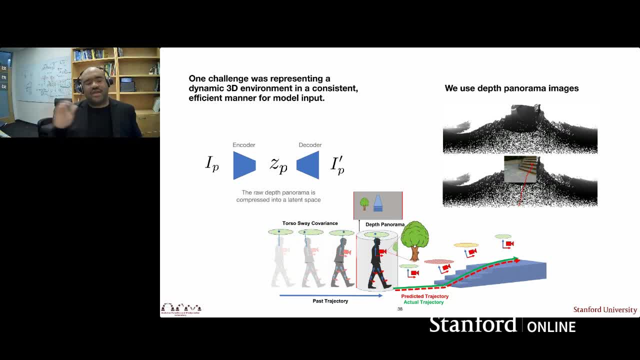 from our surroundings, And what we did was we created a panorama. So if you see this person in the middle of the screen, at the bottom there's the cylinder that encapsulates them. You can think of this as a cylindrical image where the red line can be cut and opened up. so 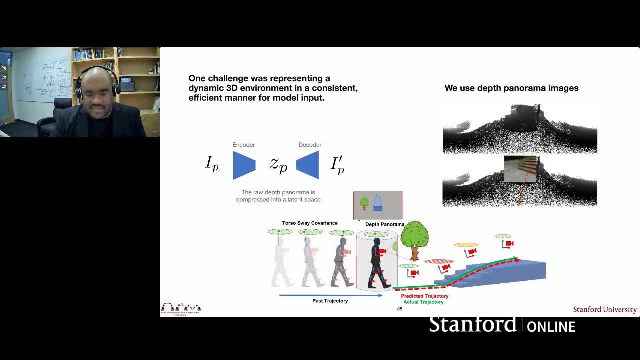 that it becomes a rectangular image you see in the top right-hand side. So whatever's right in front of you is a small area right in the center of that image which you see as the second row image on the right, And if you're walking straight ahead then that's the red path drawn in this. 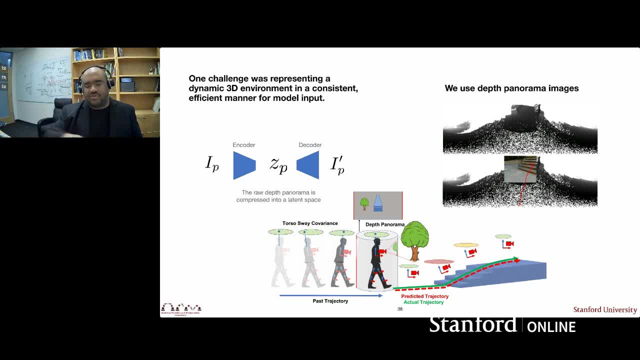 image, where your feet are at the bottom of the image, and then you would walk up in front of you based on what you're able to see, And so this was a way that we could actually efficiently represent the obstacles around us in order to provide that information to our model. 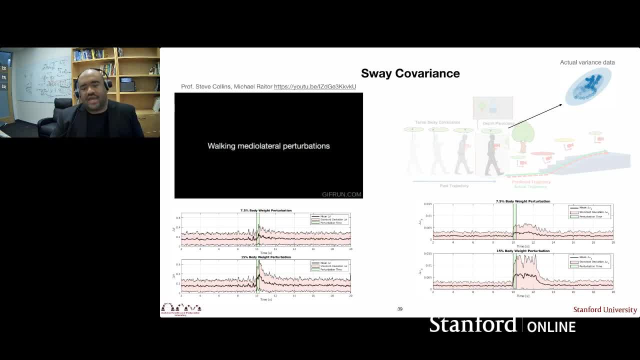 The other thing was the solution of sway covariance, And so by watching the motion of our torso, we learned that, in fact, when someone is perturbated, if you watch the statistics of how they're, if you had a z-axis pointing up straight up and you 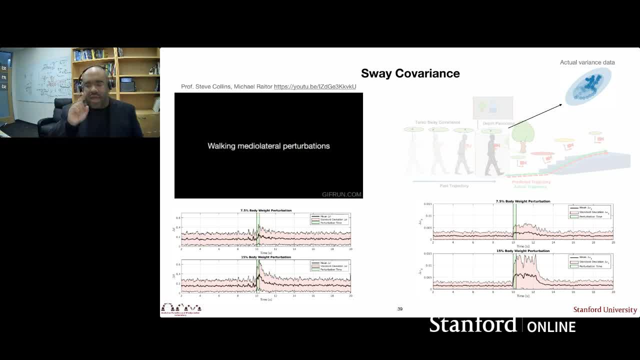 project it into the ground plane. there's going to be some natural motion that makes this sort of ellipse, this covariance. If someone's perturbated, this ellipse grows very sharply And that growth can be useful for predicting that something caused perturbation. 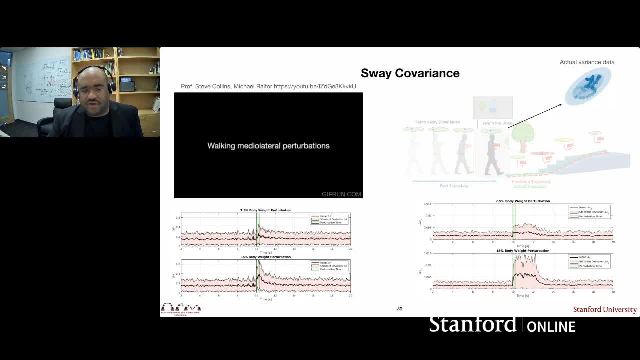 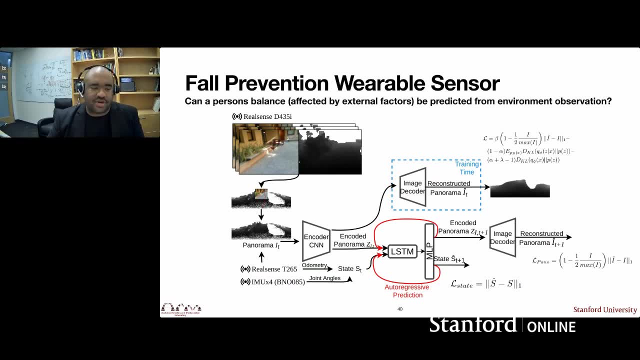 and perhaps that might be something that would cause you to fall. So this is our machine learning model that we ultimately ended up using to perform this prediction. So don't get overwhelmed by the details. I'll highlight what's important. So we have the images. 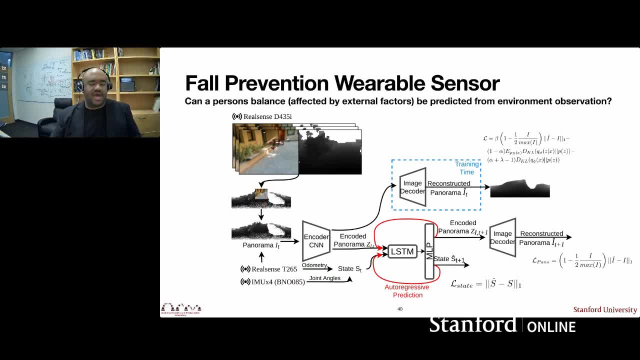 which created the depth image for our surroundings as an input. It went through this autoencoder and was represented in a latent space. that was a way for the network to efficiently model what was important in the environment as you walked through that environment, And then we had our state. We had the odometry where you were walking and joint angles. 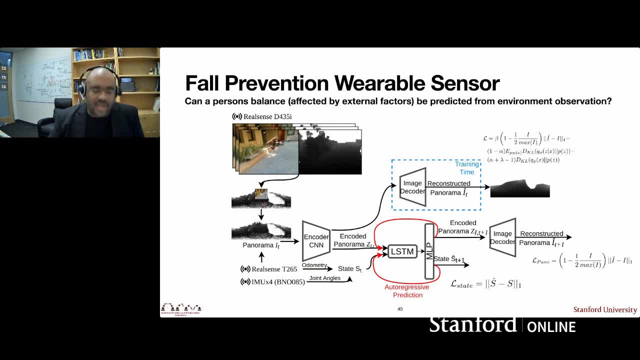 And we went through this LSTM- our long short-term memory- which is one of those recurrent networks. So it said, given everything that has happened up until now, how can I predict the next few sequences of what will happen? conditioned on the past, And then, using this, it produced how it expected: your 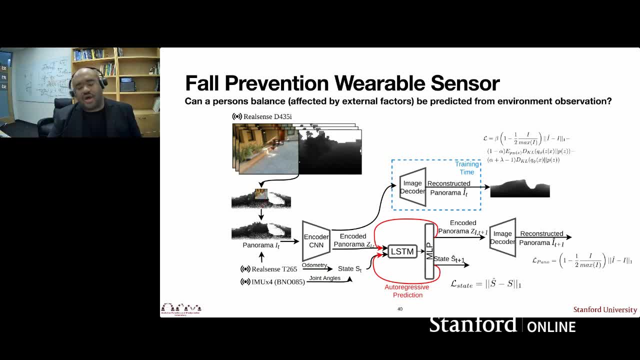 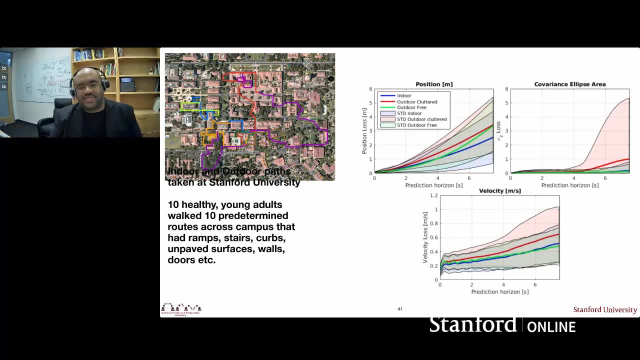 walking to evolve and how it expected your environment or your latent state to evolve as well. And so we walked in different places around campus and we collected measures for a prediction horizon of seven seconds on how well we could actually predict where you would end up. 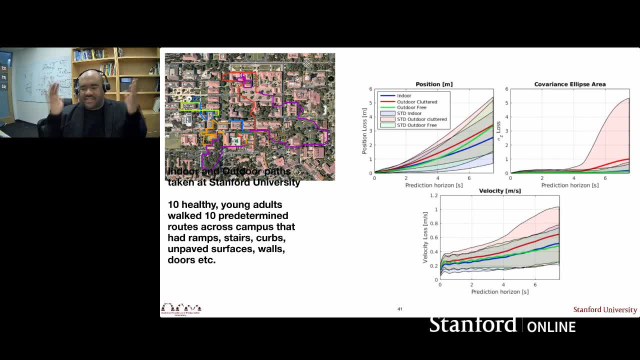 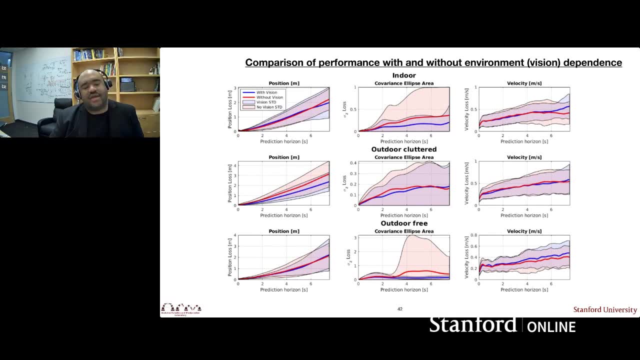 And so what we learned is if you were indoors, where it was kind of like tighter regions, it was actually really good to predict within about two meters where you would end up. So in these drawings the red line is the average line, The 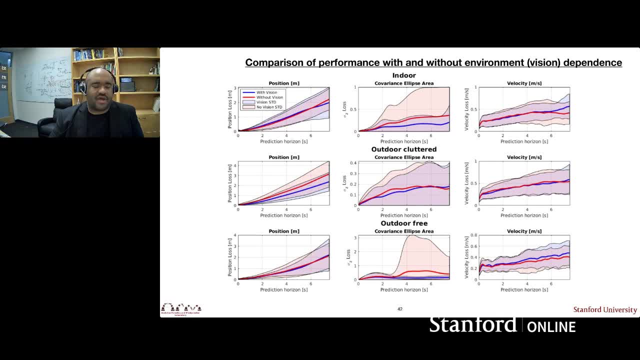 solid line is the average line, And then the colored shaded area is the covariance associated with this. So the top row is indoor, the second row is outdoor cluttered, and the third row is outdoor free, And so the point I really want to drive home here is: we could do a decent job. 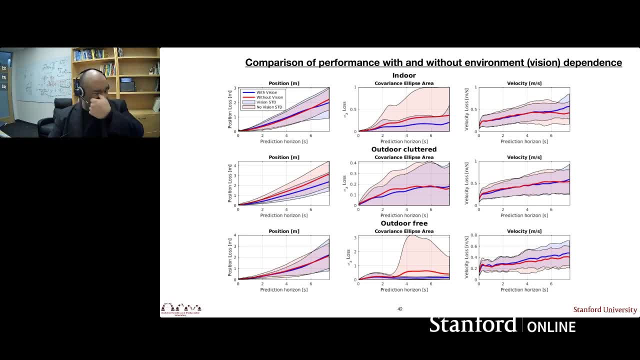 of predicting where the person will go. but there was this variance. And this variance doesn't necessarily mean our model was wrong. It just means that perhaps there were many solutions that ultimately would occur And if we only predicted one, we may not exactly be correct, because there's this distribution that a person may walk. 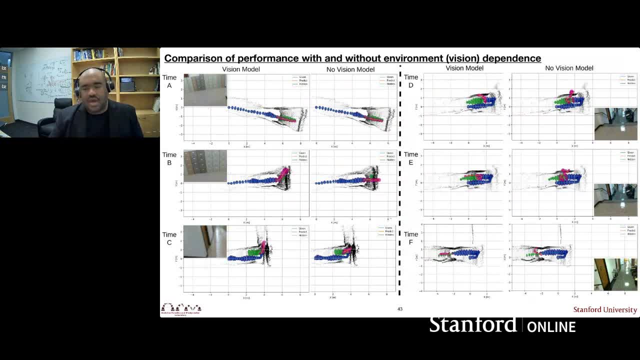 that all would be valid choices. A really cool feature- and I encourage you to again go check out this video- was actually the fact that we could do a decent job of predicting behavior in environments. So here's a picture inside of our psychology building. 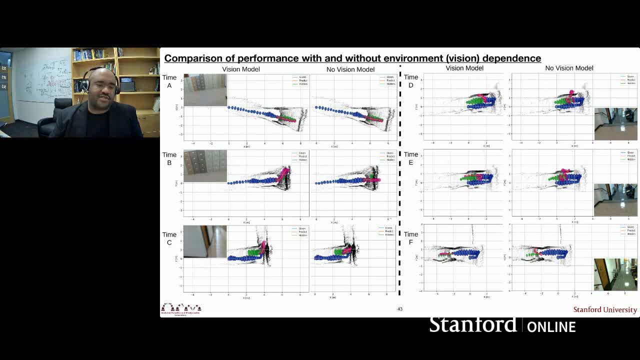 And with these sets of images you'll notice on either side of the dashed line there's, on the top row, a vision model and a no vision model for time segments A, B, C, D, E and F. If you look at the row for vision model, the blue line and its ellipses. 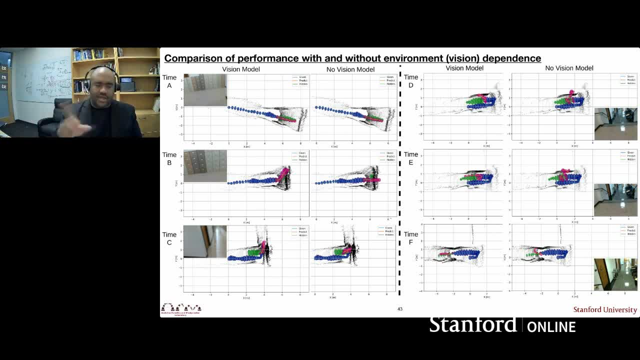 represent where you walked in the past and the sway covariance at those instances. The green line represents where you actually ended up, because we recorded all of that data and we then post-processed it to do it when we then validated it, And the red line with its ellipses indicate where you predicted you would end up and where you have. 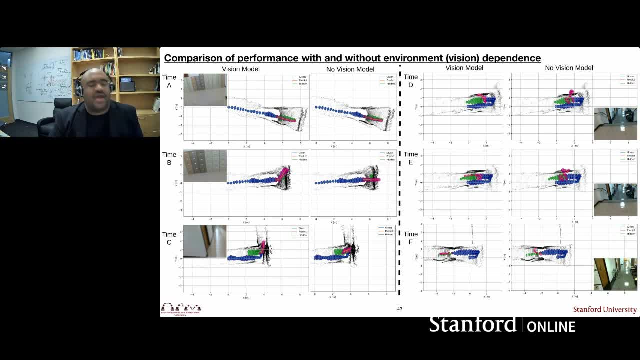 how you predicted the sway covariance of the person. And what you'll notice is, if you don't use vision, the model just assumes inertia. It assumes if you're walking in a particular way, you're going to keep walking, because that's all it has access to. But if you incorporate 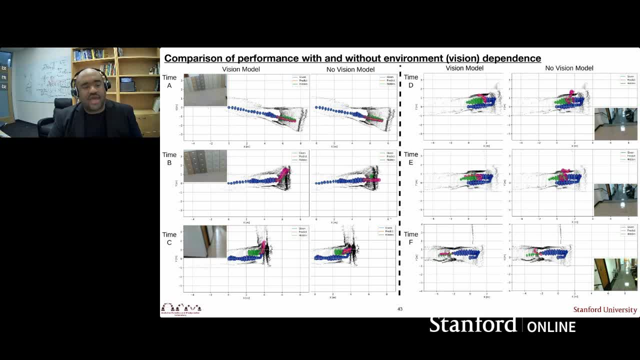 conditioning on the environment and pass data of people walking, it begins to learn that it can't walk into walls, that there's likelihood of you turning down walkways when it's available, And then, given how you're orienting your body, you may walk in a particular way and, given your speed, 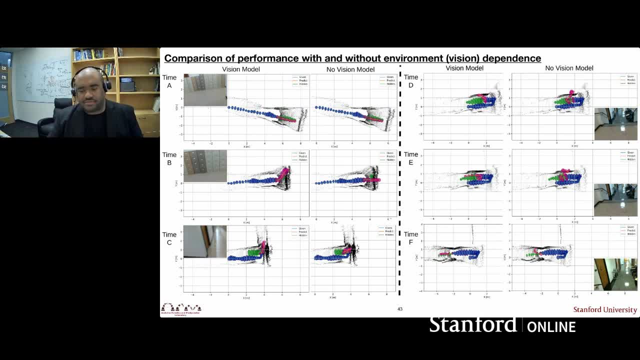 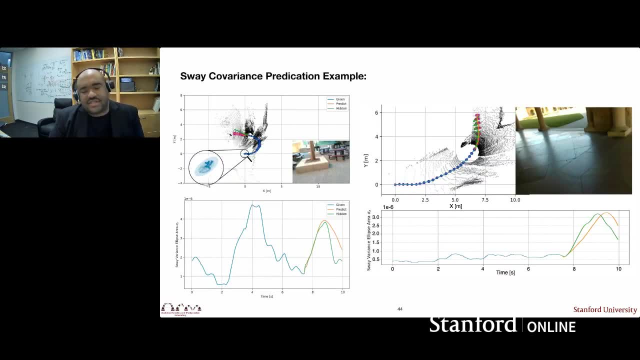 you can predict how fast you'll walk in the future as well. Another really cool feature here was, as you walk in particular environments, there was actually a correlation in your sway covariance as you walked in those zones. So here's a picture of my graduate. 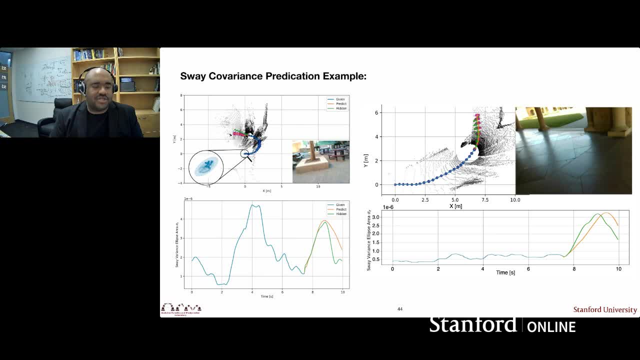 student. He's walking around campus And what was interesting was, when he took sharp turns, his sway covariance changed in a particular way And, after being exposed to that type of data, the model was actually able to predict the motion of his torso, given the path that he was going to walk. 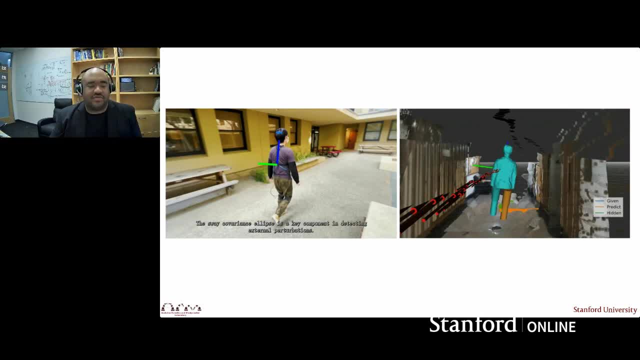 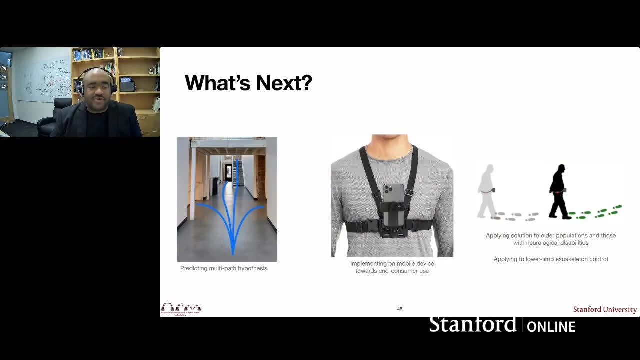 And so, again, these are some really cool videos I encourage you to check out. You can actually see in real time that motion of the torso, as well as the sway covariance as they walk through an environment- Some future directions for this. Well, we have that covariance. It wasn't perfect. 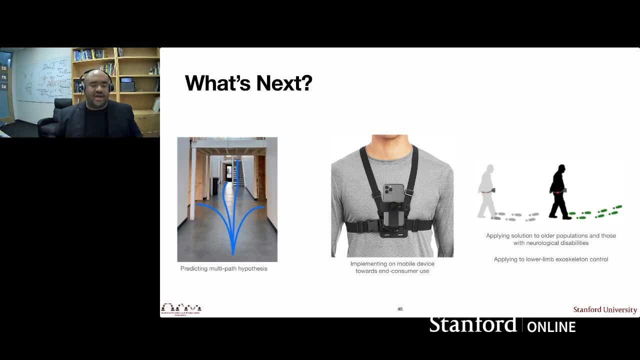 So what if we wanted to predict multiple trajectories And perhaps the sensor system? the system that we showed you is not cool enough for people to wear. It would be better if it could perhaps be a smartphone, And then, down the line, we'd like to also actually help populations that. 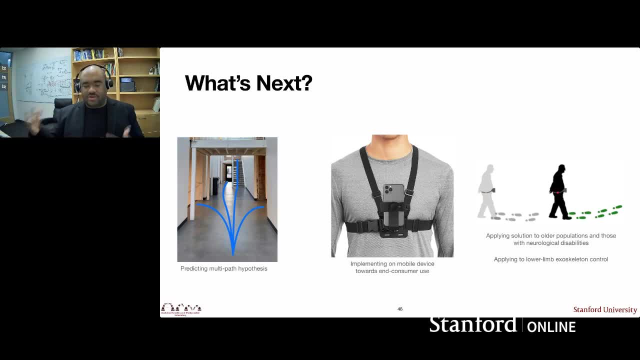 could use this. So this could be older populations or people with neurological disabilities. Could you outfit them with the sensor, collect their data and then make this system work for them And perhaps use this also in lower limb exoskeleton control, which my lab is excited to collaborate with? 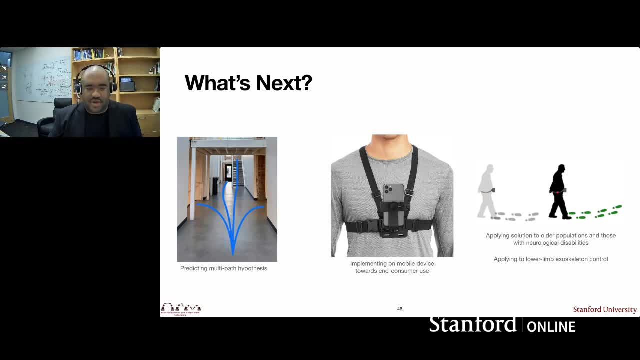 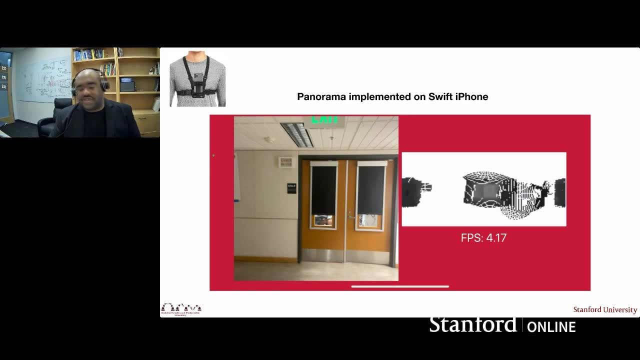 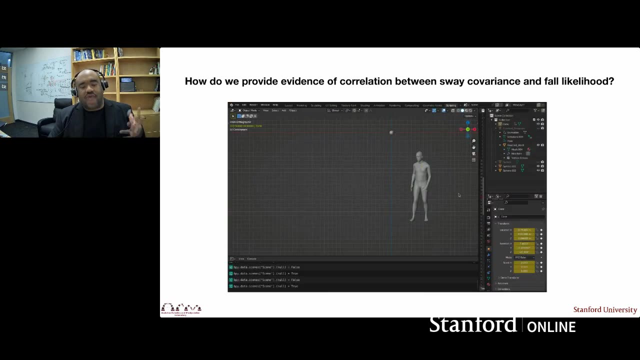 Professor Steve Collins here in the Mechanical Engineering Department at Stanford as well. So we've implemented this on a smartphone. We are actually able to get really good depth representation data. My student is also trying to improve the ability to estimate sway covariance. We have this software called 4DHumans that's able to extract the pose of the person. 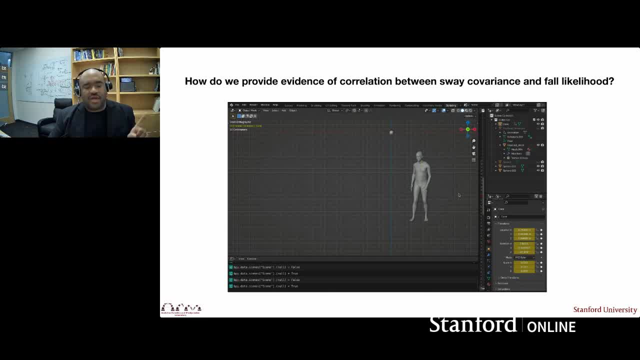 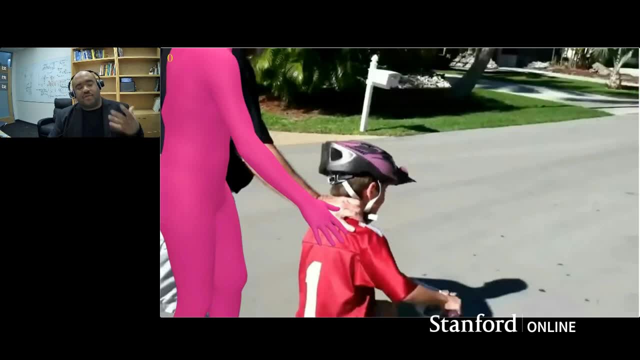 and then we can actually monitor their sway as they walk, And then we can actually collect videos from the wild where we see instances where people fall, and we can learn if our parameter is actually useful in a way in predicting whether those falls might occur. 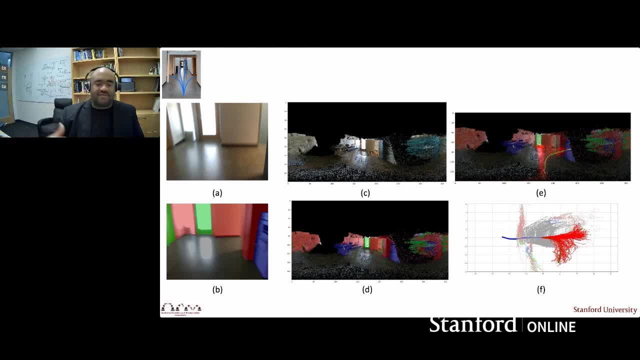 And finally we're able to say: well, given the fact that we might want to predict multiple paths and environments, we can use diffusion models to actually predict those multiple hypothesis paths. So here we use a segment, anything framework from Facebook to actually partition doors, walls. 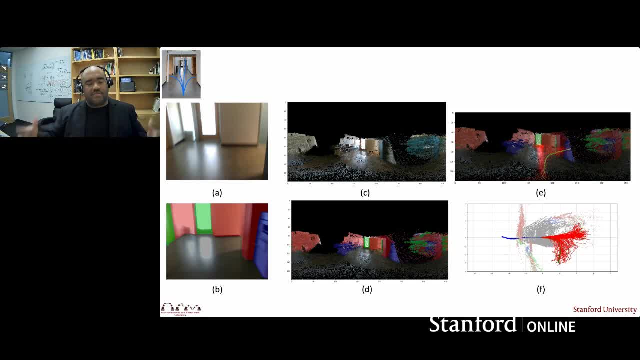 obstacles ground and then, with this, watch the data where people walked and then predict multiple hypothesis of where they may end up. So here you see two distributions of paths: some that lead through this doorway, others that make a turn, and both of those. 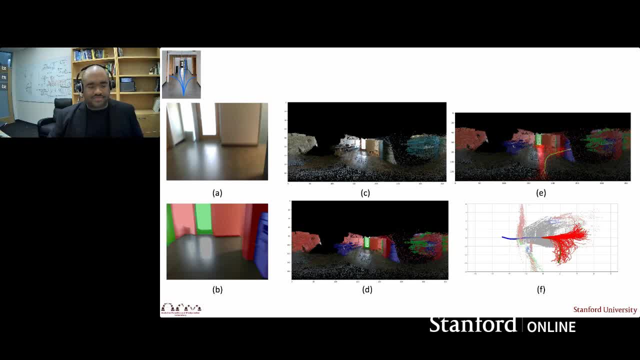 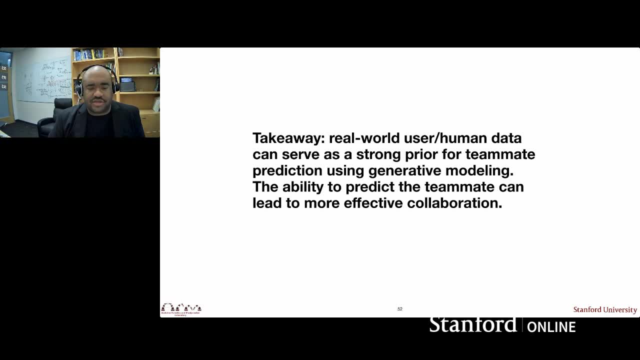 are actually valuable outcomes. So the takeaway I want to leave you with today is that real-world user human data can serve as a strong prior for teammate prediction through generative modeling, and the ability to predict the teammate can lead to more effective collaboration, And I will end with that. 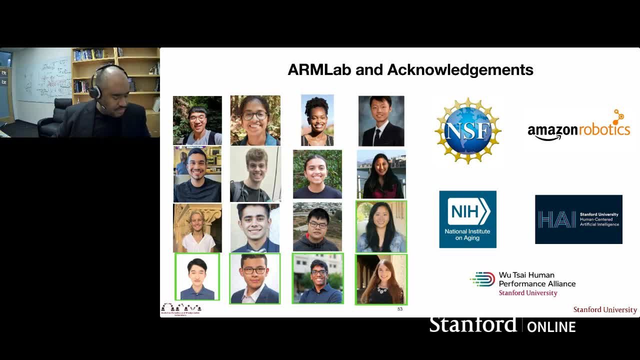 Thank you very much, TESSERA MONROE- Tessera Monroe. thanks so much. This is Really interesting and a very insightful presentation. You and your lab are doing some really great work and it was really great to have you share that. 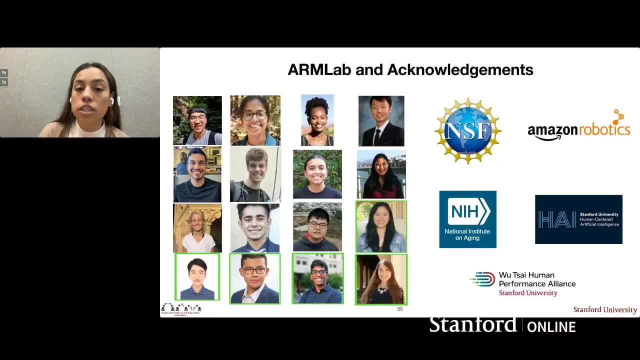 with the audience today. Now let's get into some questions. Bill, did you want to kick us off, And then I will take a look at what we have in the Q&A. BILL WELDON- Well, we have a limited amount of time. 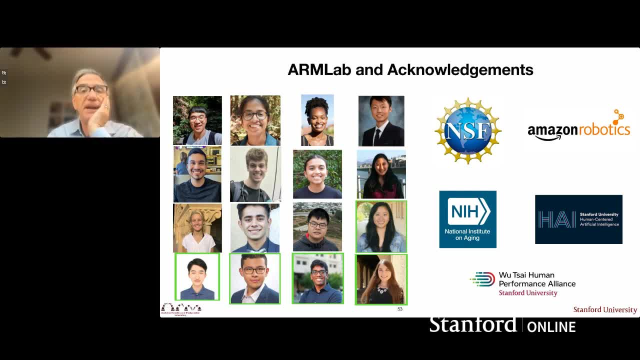 So I think I'll just have one question, but let's jump into the Q&A. Monroe, you mentioned some things about fall detection or focus. TESSERA MONROE- Yeah, Yeah, BILL WELDON- And I'm going to start. 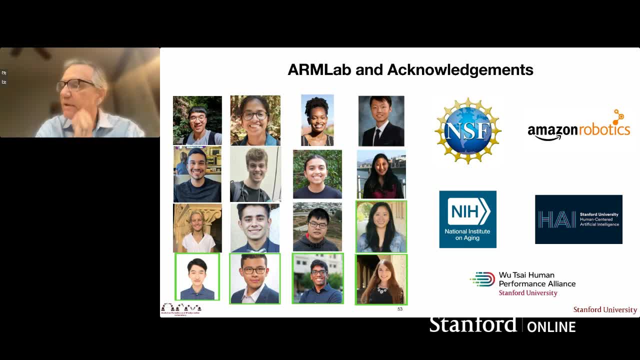 with folks who have disabilities. Can you talk a little bit more about what your lab is doing with these predictive models that might be useful for folks that have either limited mobility or other disabilities? TESSERA MONROE- Yeah, So two of the ones that I mentioned today particularly. 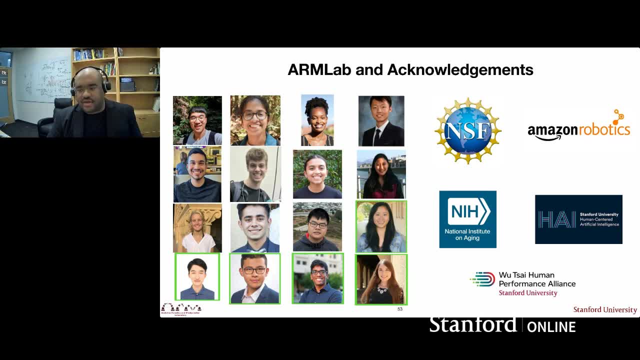 included the intelligent prosthetic arm and the other, like the fall prevention sensor which you just mentioned. I think in both cases, the question that we're asking is is one of intention estimation- right They're either. in the case of the intelligent prosthetic, 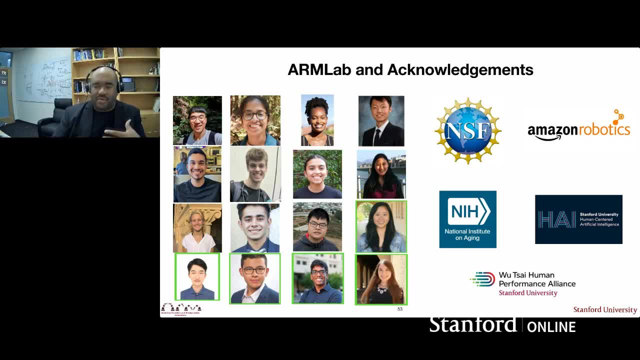 the person does not have an ability and we want to endow them with that ability. But they have the ability to give us some sort of input. But if you're trying to control these systems, the degrees of freedom that you need to control. 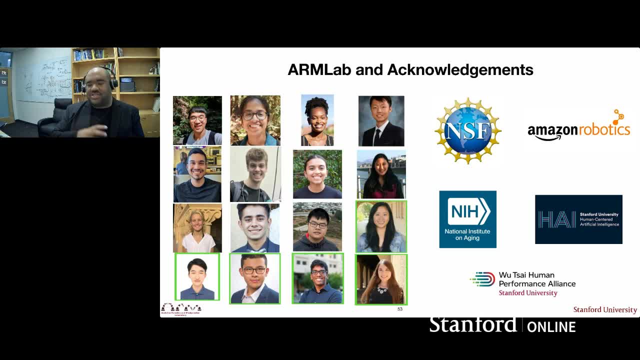 are so high and complex that it's very difficult to extract that low-level control from the person. TESSERA MONROE- Right. BILL WELDON- So if we can bring robotic autonomy, we can do that. TESSERA MONROE- Right. BILL WELDON-. So if we can bring robotic autonomy, we can do that. TESSERA MONROE- Right, BILL WELDON-. Right, BILL WELDON- Right, TESSERA MONROE-. So if we can bring robotic autonomy, 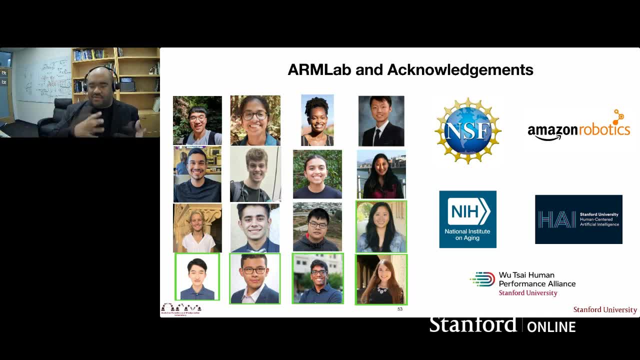 where a robot knows how to do a task and then couple that with clever ways of reading the person, estimating their intent, then we can return, hopefully, some of that ability, some of that agency for them to do particular tasks And, in the case of the fall prevention sensor. 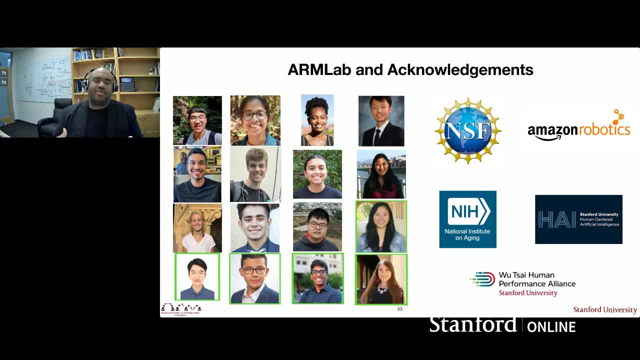 this is augmentation, So we assume that the person is capable, but they could use some help to avoid some unfortunate outcomes, And this could again be in fall prevention or in exoskeleton control. TESSERA, MONROE- Right. 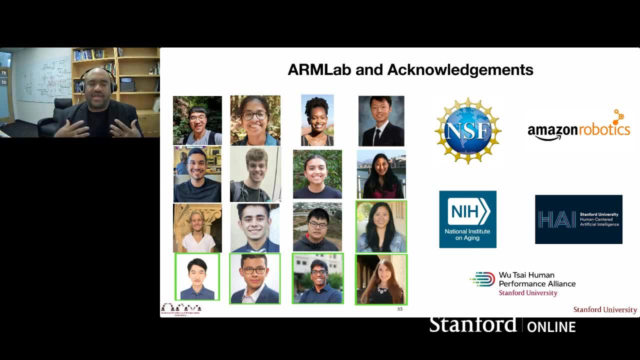 BILL WELDON- The idea here is, you may not necessarily be replacing their ability, but your ability to predict and assess and predict risk becomes useful in protecting or helping these individuals. TESSERA MONROE- It's just fantastic And I have a sense from your talk. 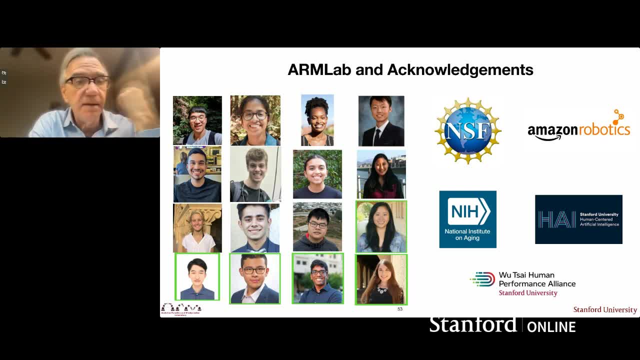 that we're right on the edge of some amazing new capabilities, either to augment human capabilities or to replace things that, for whatever reason- age or something like that, Or disease or something- has caused us to have a disability. Annette, do you have some questions from the audience? 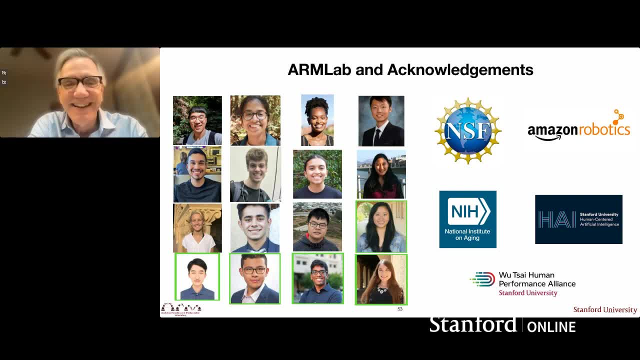 I'm sure they are full of questions, ANNETTE GORDON- I do. There are a ton, So I will try to get as many as we can. But to kick us off, Professor Monroe, as we progress towards machines understanding human intention. 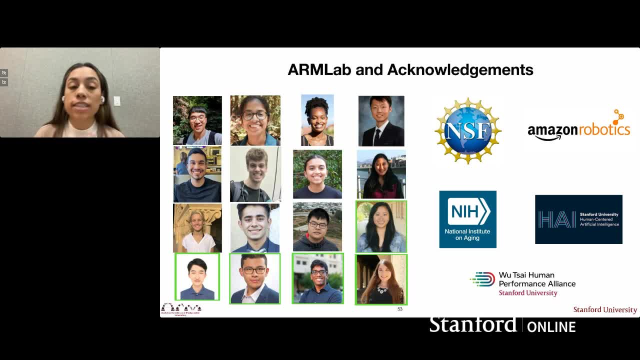 what potential positive and negative impacts could this have on society And how can we ensure responsible and ethical development in this domain? ANNETTE GORDON- That's a great question. I would start off with the sort of positive, by really just emphasizing need. 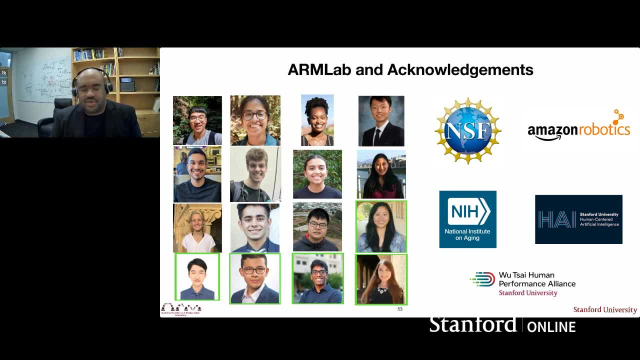 I think to date, many times the conversation with robotics and robotic autonomy is concern around replacement, But the goal of robotics is to improve human life, And so that doesn't always necessarily mean a robot replacing a particular task If the task is very dangerous for people. 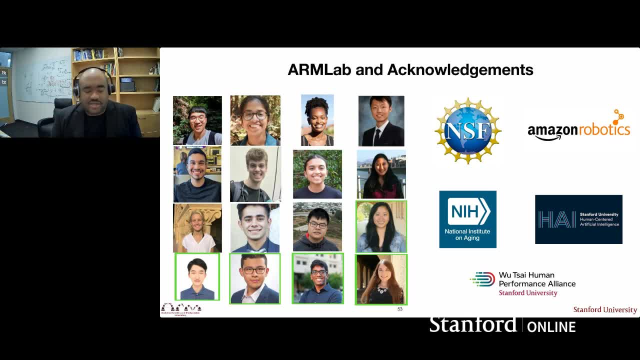 and people are getting hurt or they're being mistreated, then perhaps a robot should be replacing those instances. But if that's not the case, then maybe augmentation is the answer. How do we make people more efficient? And so I think, thinking about examples in assisted living. 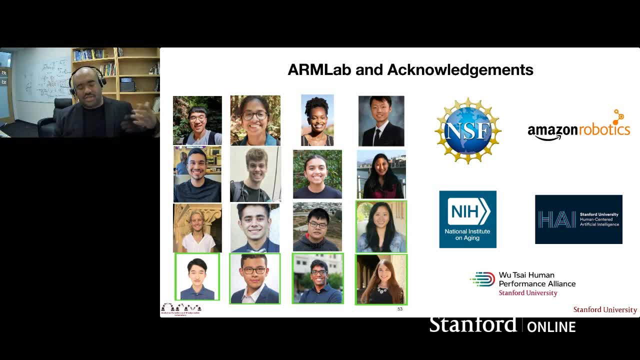 you could have robots that could work with people who want to live in their house longer. Maybe they have small issues with dexterity and other things, but they're cognitively all there And they could hopefully live on their own a little bit longer. 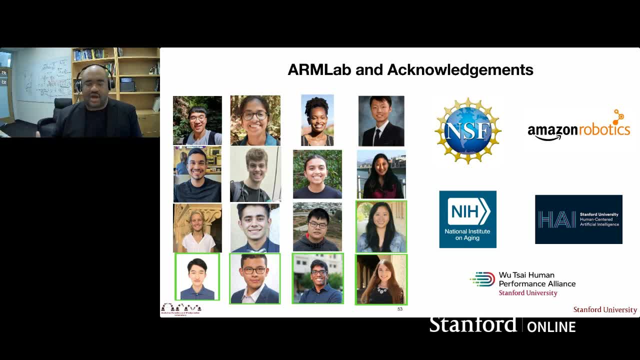 with the aging population worldwide. Having these types of systems that could help in that way would be extremely helpful, And you can think of other instances in agriculture in terms of helping with sustainable foods, having robots that could work along farmers to achieve those things. 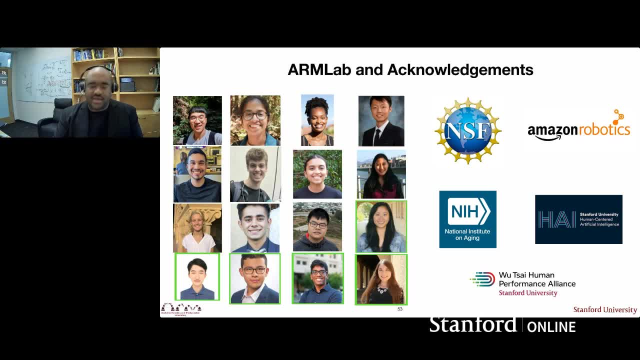 You could think of the elderly population, as I mentioned, manufacturing, making sure that's humane, effective, while not necessarily diminishing output, are all very good potential outcomes. Thank you, And I think, as with every engineering tool, ethics is important. 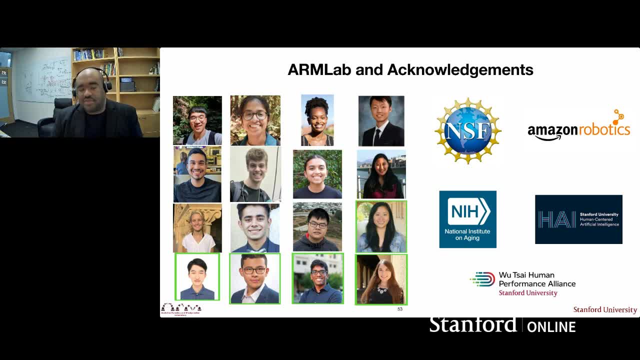 And there are ways that these things could be potentially abused or misused. One that immediately comes to mind is: I think at some point we want to make sure that these solutions are democratized. They should be accessible to everybody, And so it would be great to say I. 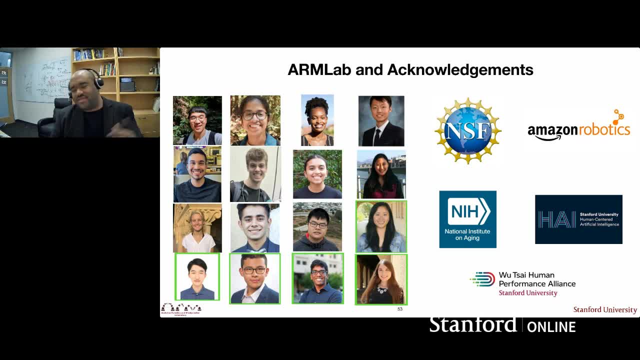 have this robot that has all of these capabilities. I would love to say, if I put this robot in an old, I would love to say, if I put this robot in an older person's home, maybe there's a flat rate that they have for this. 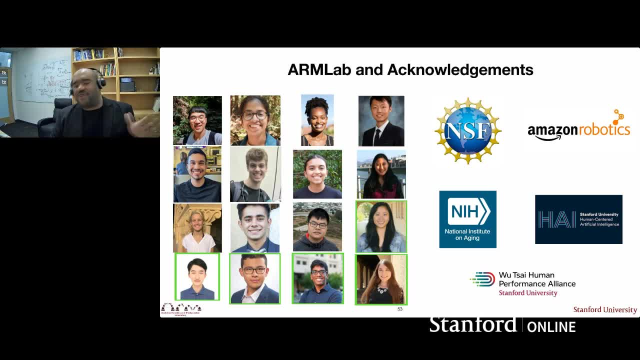 And there should be a level of functionality that they should not be nickel and dimed for. Oh, my robot can make tea, so you have to pay a subscription fee of $10 a month if you want it to make tea for you. If it knows how to make tea, it should make the person tea. 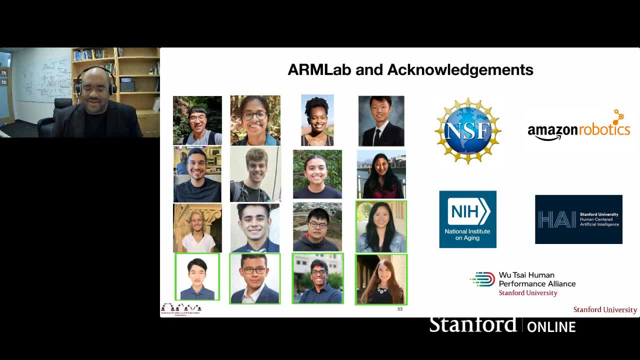 I think, making sure that the fundamental skills of these systems are democratized so that there's accessibility and usability and that we stay on track for net positive effort. Again, I think these tools are very powerful, Even more fundamentally than the robots. 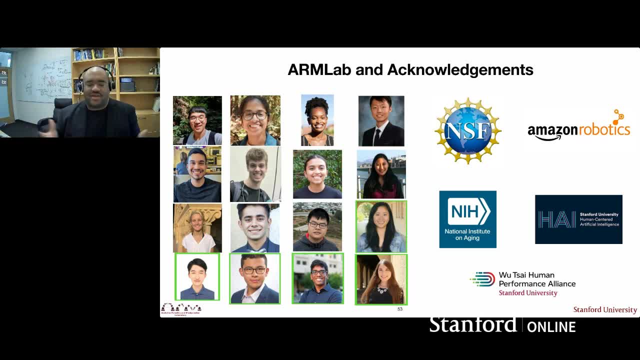 the power of prediction is itself a very incredible thing. We predict the weather and it leads to us being able to protect ourselves, But everything again has the ability to be misused. So I think there is an idea of fundamentally thinking. 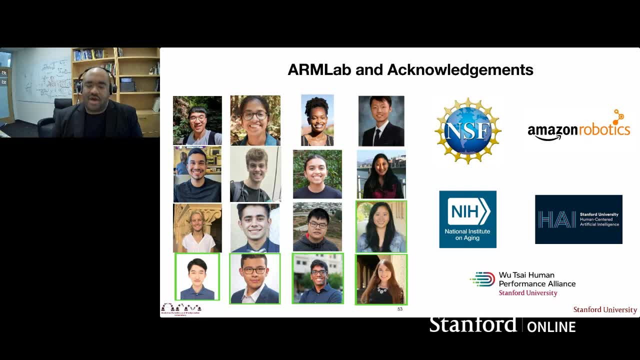 it is our responsibility to make sure that the solutions we develop are helping people and not harming them And at some level, with every powerful tool, it does become on the honest of the developer to make sure that they're being used in responsible ways. 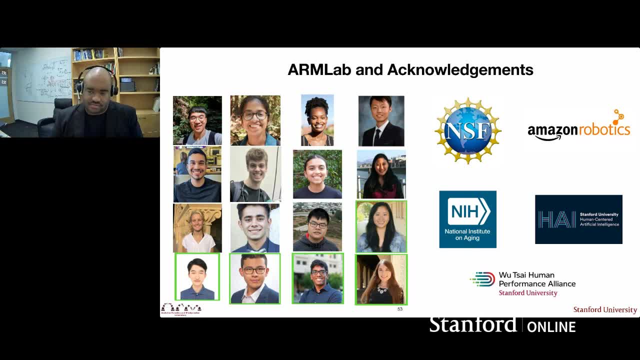 and society to hold people accountable when they're not. Yeah, that's great. Thank you so much for those insights. I think we have time for about one more question. So I know you touched on this a little bit in the presentation, but one of our participants. 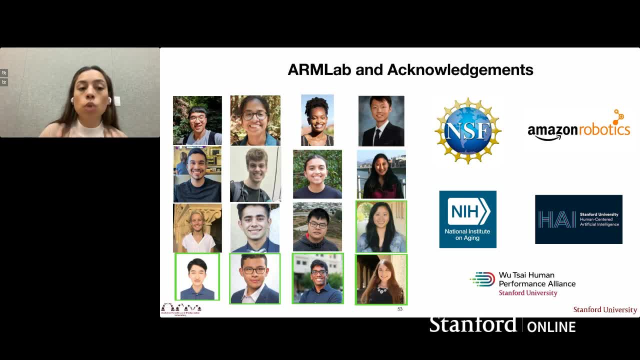 is interested in kind of expanding more around. what role does artificial intelligence and machine learning play in advancing the field of human-robot interaction, specifically in enabling machines to understand and adapt to diverse human intentions? That's a great question. So I think machine learning again. 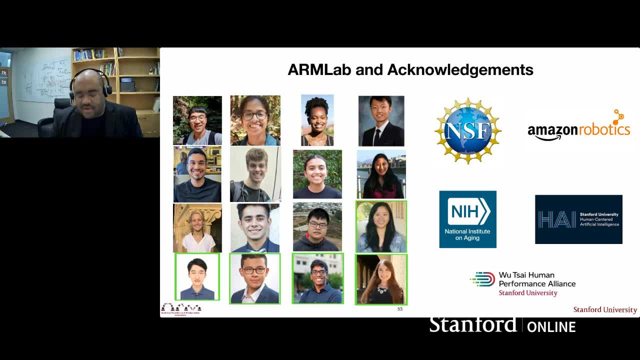 plays this really fundamental role of allowing us to model stochastic processes. If you put an input in and you expect a single output, that's an analytical description. that can be very useful for things where the rules are very defined. But data science is becoming very popular. 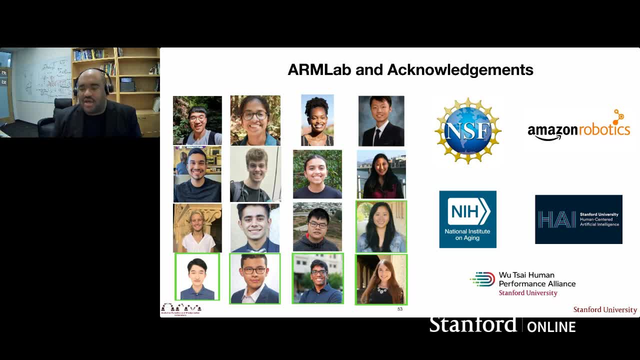 because the real world is often very hard to model and also very noisy. However, there's a significant power of statistics to be able to understand the distribution of particular outcomes, And machine learning and AI is that tool that sits on those statistical principles in order to allow us.